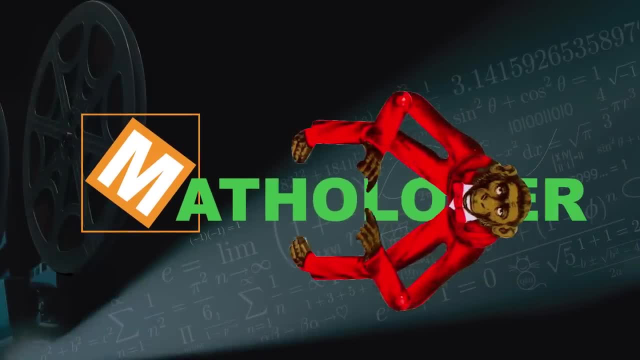 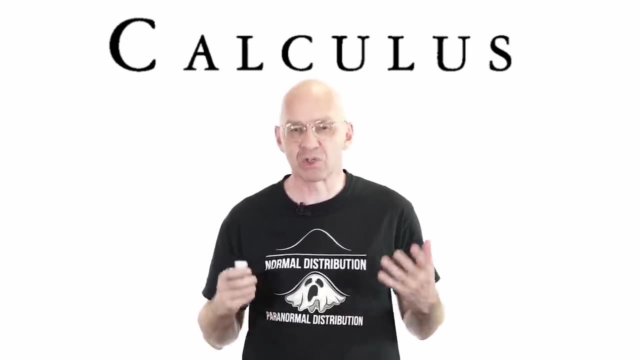 Welcome to another Mathologer video. People are always going on about how hard and complicated and how terribly high level calculus is. That's actually only partially true. When you look at it in just the right way, the core of calculus is actually very simple and straightforward. 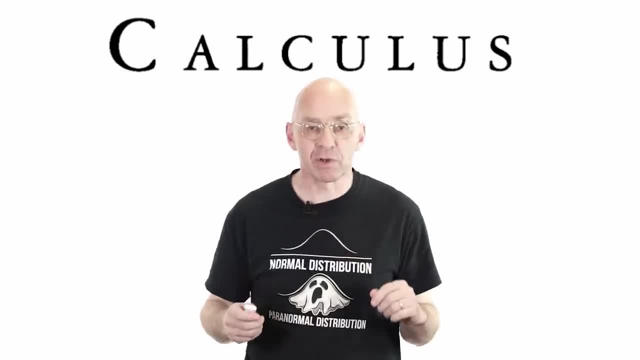 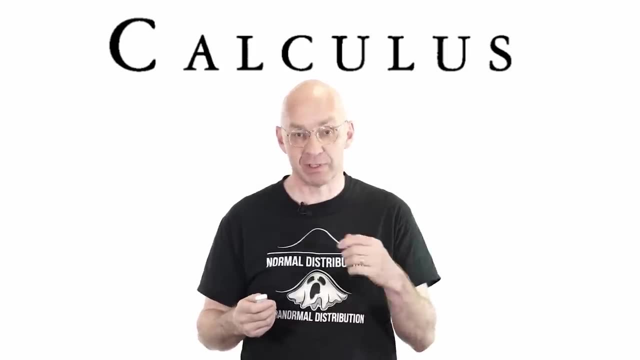 really not much harder than basic algebra. In fact, when I was only 13 or 14 years old, I got introduced to calculus via the book Calculus Made Easy by Sylvanus P Thompson, a book which is all about showing how easy calculus can be. It's an amazing book and 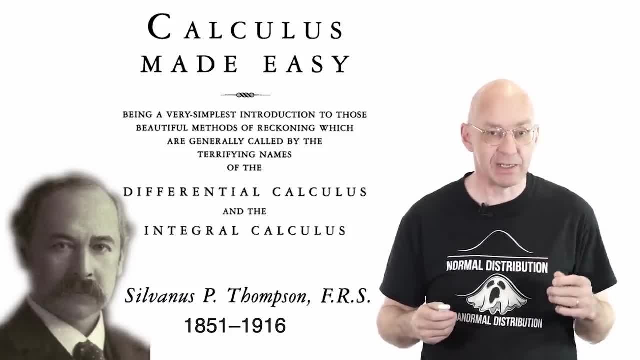 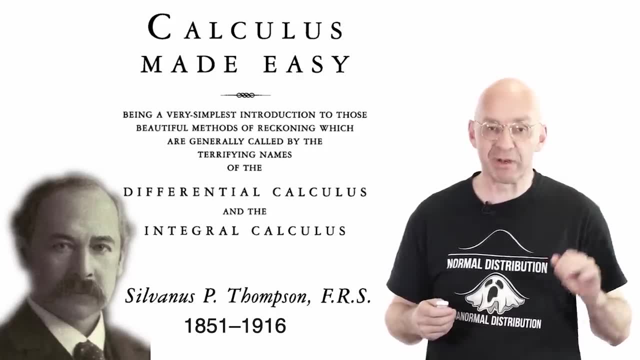 really worked for me, And I'm not the only one. Published in 1910,, this book went viral pretty much straight away, is still in print after more than a century and is sold. wait for it over a million times. 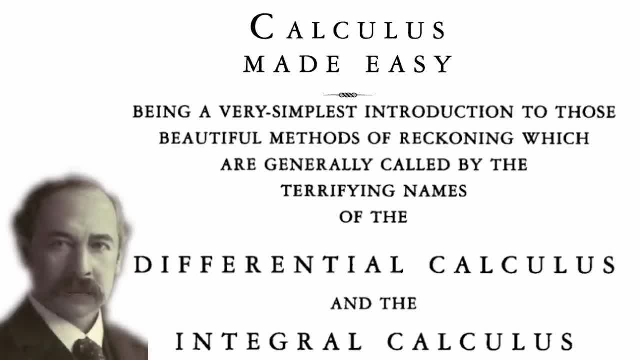 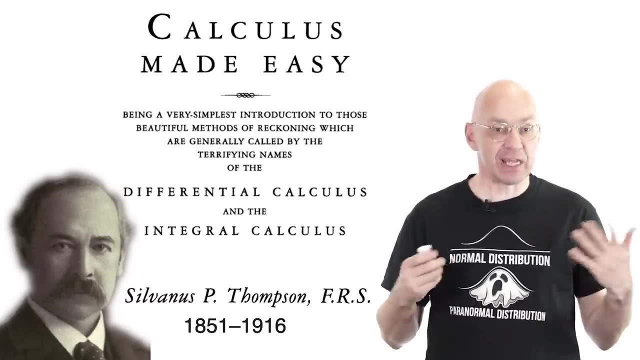 Calculus Made Easy, being the very simplest introduction to those beautiful methods of math, methods of reckoning, which are generally called by the terrifying names of the differential calculus and the integral calculus. Terrifying names, not something you'd expect to read on the cover of a calculus book. It's. 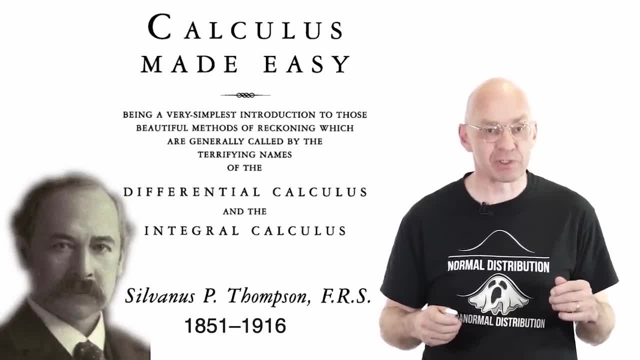 an unusual book in many ways, and the way calculus is explained in this book is also quite different from the way it is explained in regular textbooks both then and now. I'll put a link to an online version in the description. Well, I've been explaining calculus myself for the better. 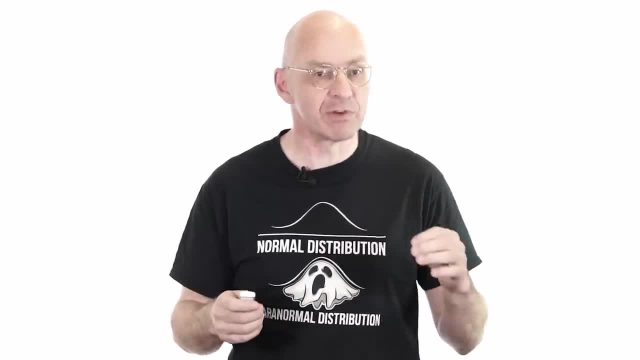 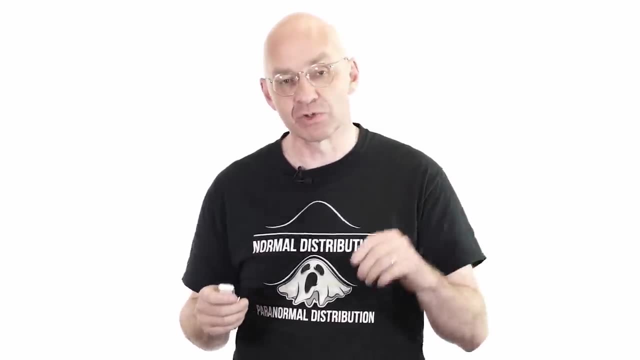 part of my life, and what I'd like to do today is give you my own version of calculus, made easy in this video. Of course, there are lots of calculus videos out there, but, as usual, the aim of a Mathologer video on something as done to death as calculus is to present. 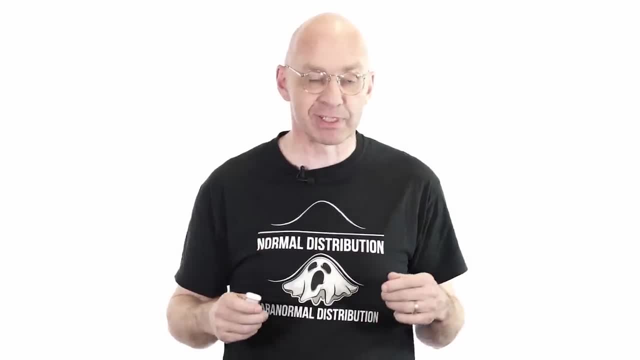 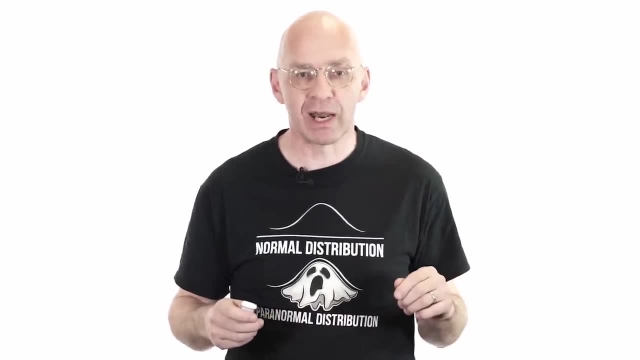 a fresh and optimal take that both novices and experts can enjoy. Okay, so here's what I've got planned for you. In the first part of the video, I'll show you the that your car is actually a calculus machine, and I'll show you how you can perform those. 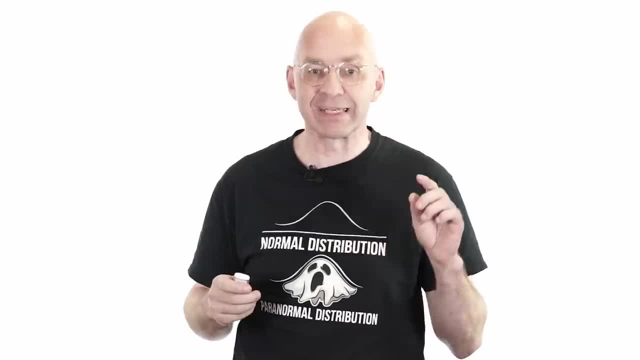 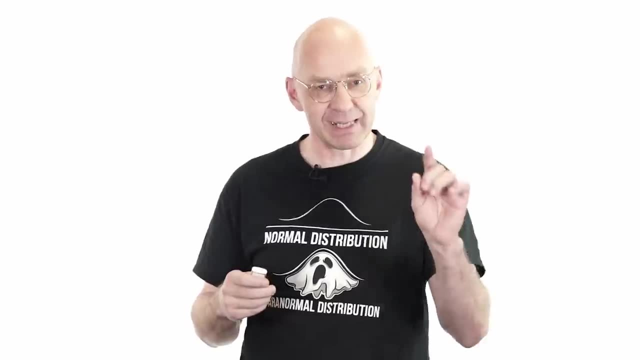 two terrifyingly named methods of calculus- differential and integral calculus- by simply driving around and repurposing the speedometer and odometer of your car. In the second part of the video you'll find out that the core of differential calculus is such a no-brainer. 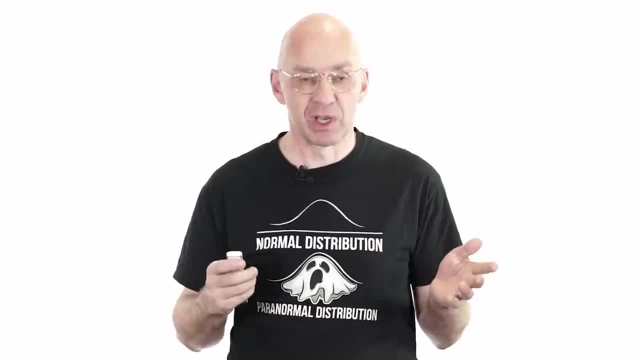 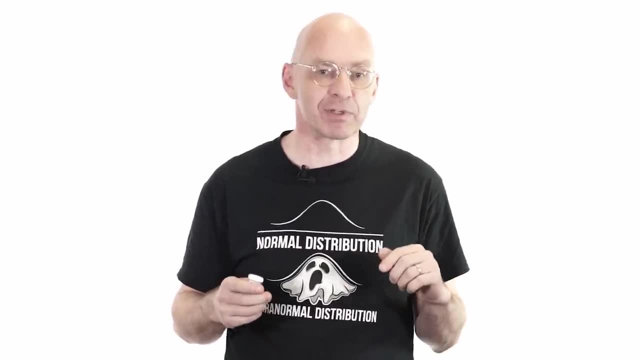 that you can teach it to a monkey. Pretty miraculous, really. On the other hand, the core of integral calculus is far from monkey. see monkey do. Still, there's lots of easy and powerful stuff there too, which we get by putting differential calculus in reverse. 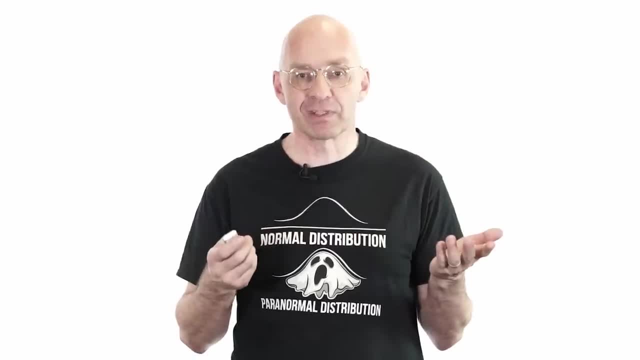 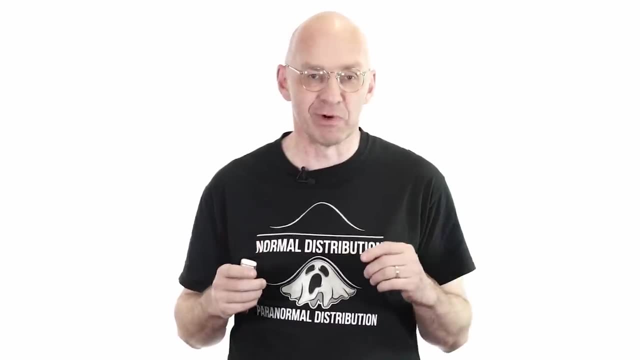 We'll do that in part 3 of the video, And I'll finish off with something I've been meaning to put together for a long, long time: a 5-minute animation in which I derive ALL the most important formulas of calculus along the same lines as it's done in that amazing 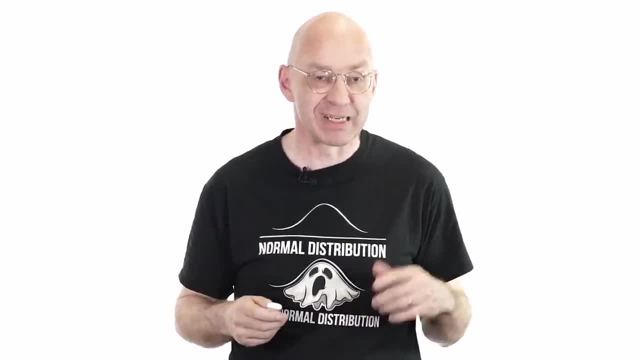 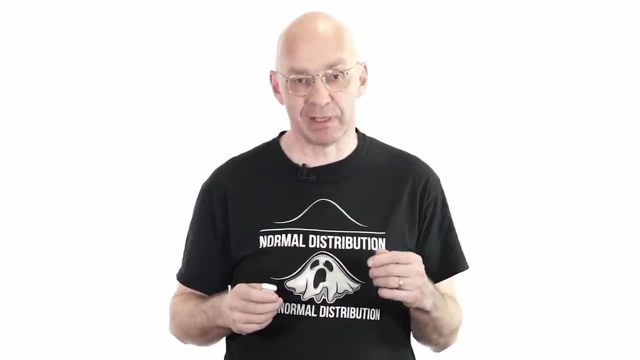 book that I just mentioned: 5 minutes for everything important. This miracle is made possible by an ingenious way to capture calculus in symbols – courtesy of the great Gottfried-Wilhelm Leibniz, one of the inventors of calculus. That's all that dy dx stuff infinitesimals. but. 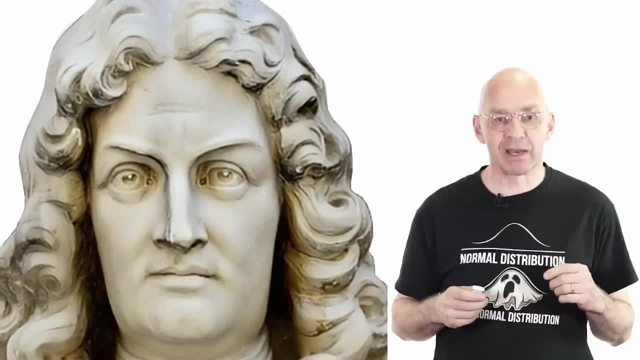 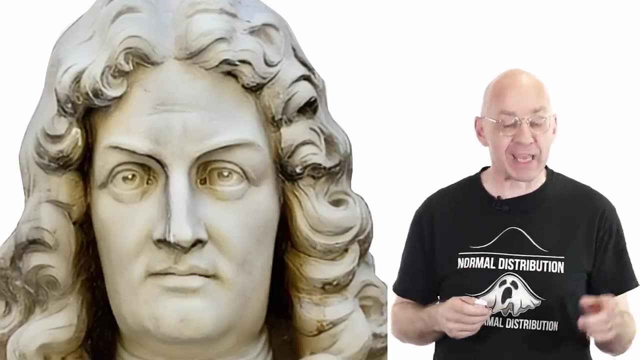 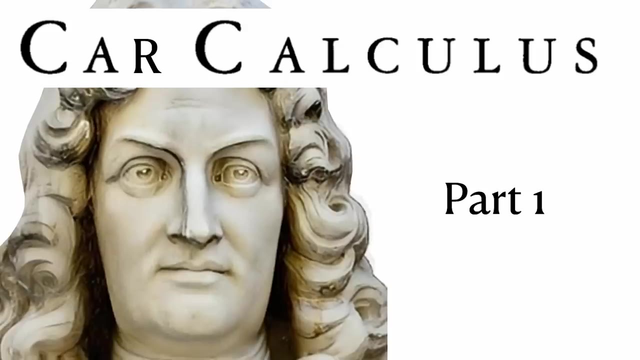 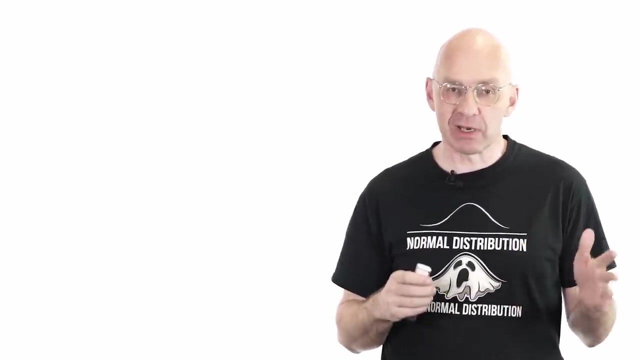 on steroids. This video is by special request for my kids, Lara and Karl. Karl is actually there in the background looking at me. It is therefore also dedicated to them. Are you ready for a wild ride? Okay, then let's go. Hmm, wild ride. Well, let's imagine that we are cruising along in the 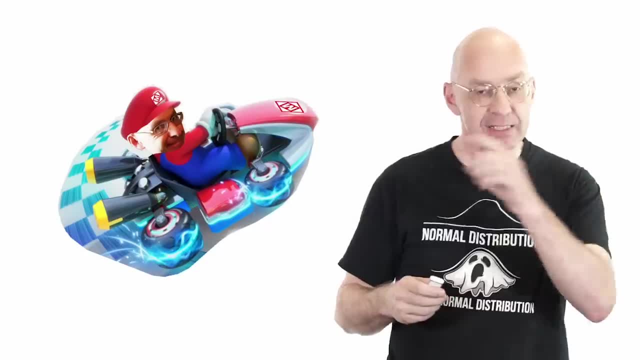 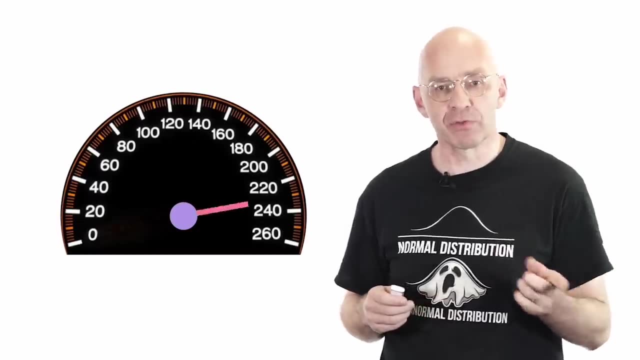 Mathologermobile on the Autobahn in Germany. Let's have a look at the speedometer. Okay, speed going up, speed going down and speed going through the roof. But remember: no speed limit on the German Autobahn and so no 260 kilometers. 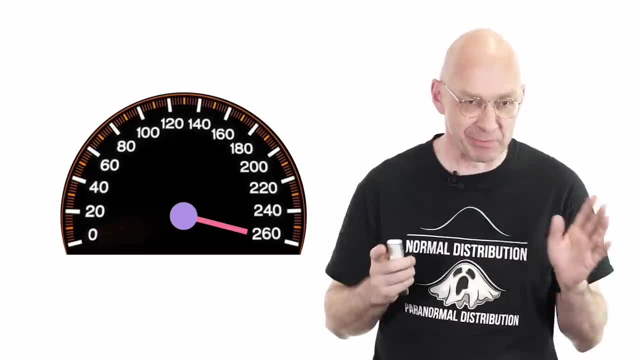 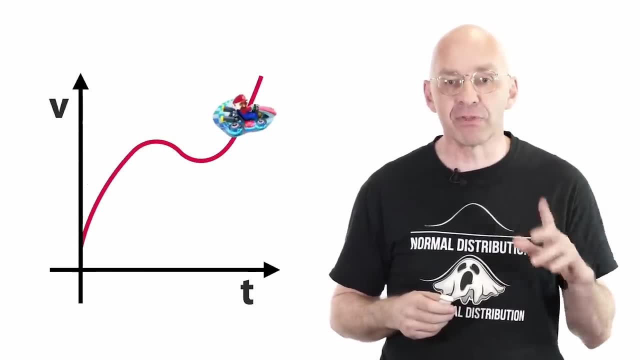 per hour is not a problem. I do this every time I go back. Okay, at some point let's start plotting speed versus time There: speed going up, down and through the roof. Now how can we translate the speed time diagram into a distance time diagram which records how? 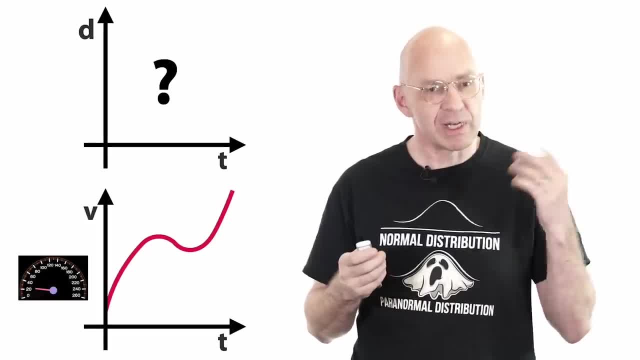 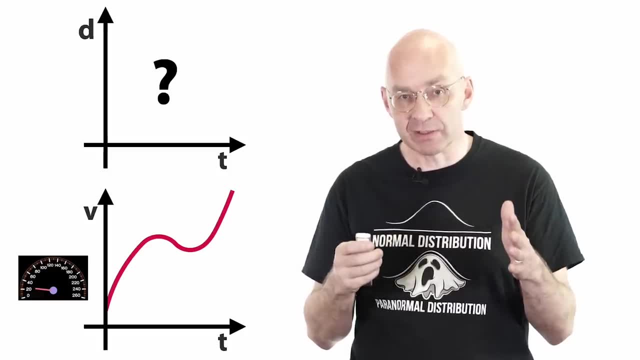 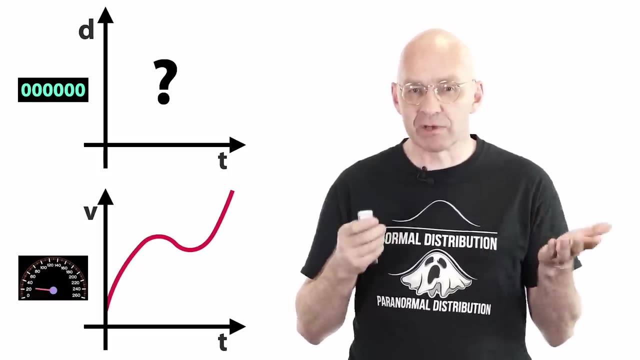 far we have traveled since we started recording. Very natural thing to ask, right? Well, basically, what we're asking is this: How can we translate the speedometer reading into the odometer reading? Obviously, this is translations hardwired into our car, but how does this translation actually work? 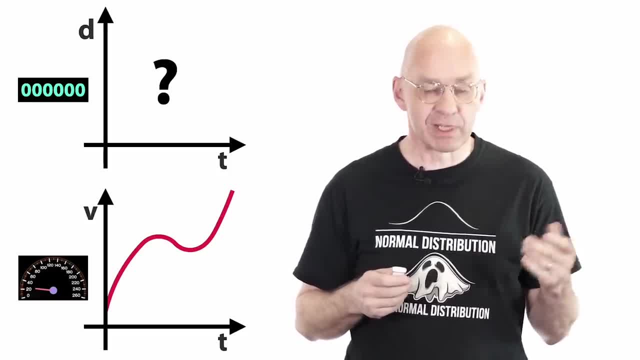 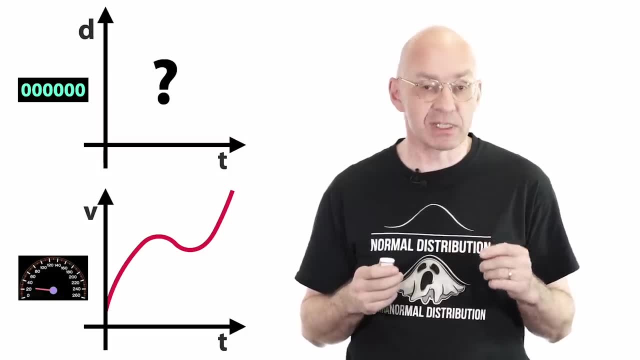 Well, if you've never seen this before, I'm not going to blame you if you say no idea. Well, to get some feel for what's going on, let's look at the simplest case where we're cruising along at a constant speed. V Now, constant speed corresponds. 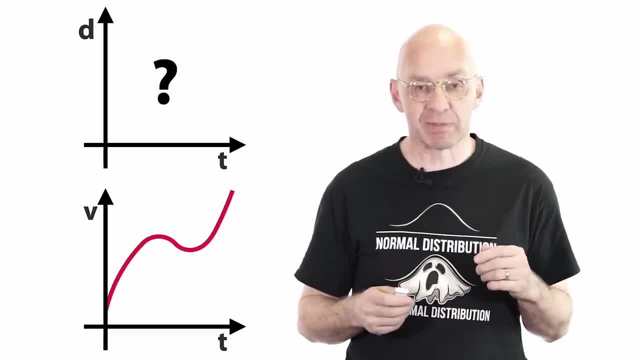 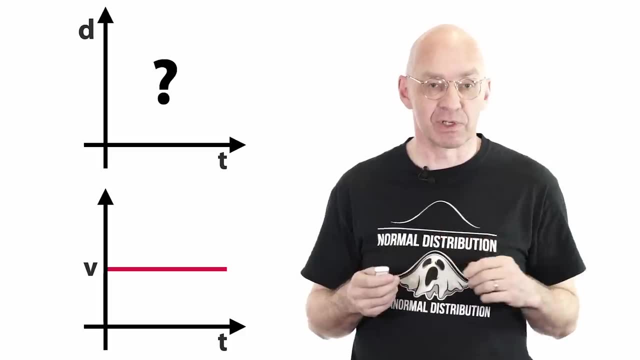 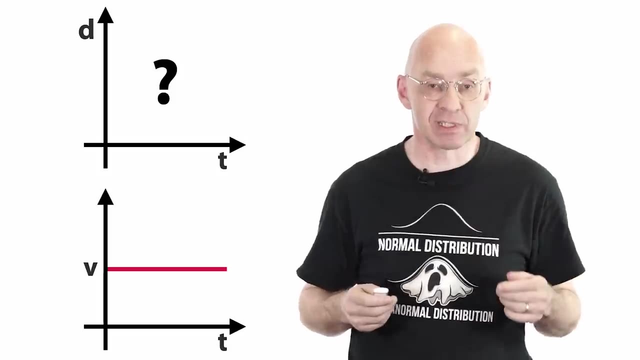 to horizontal line at height V in our speed time diagram. There, constant speed. In the case of this simple speed time diagram, we actually know what the corresponding distance time diagram is. It's given by the kindergarten formula: distance equals speed, times, time, And so the distance time diagram we're. 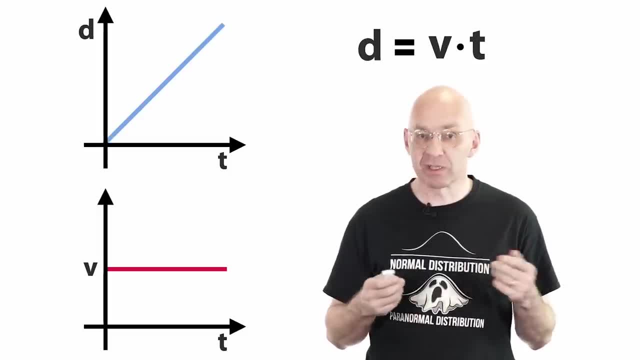 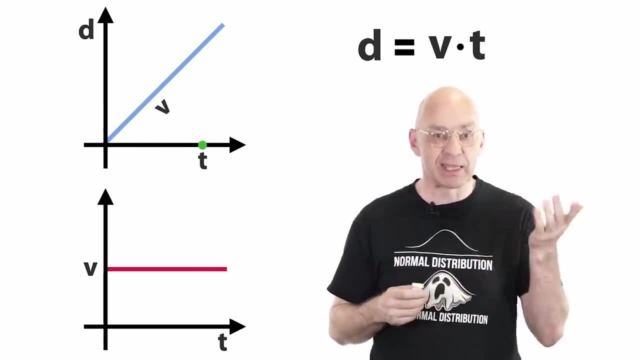 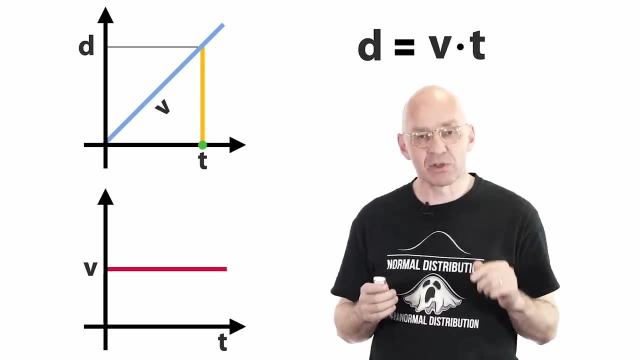 interested in looks like this, with V being the slope of the blue line. Easy peasy, And so the distance traveled at time t is just the length of this yellow segment. On the other hand, and this is a crucial insight, our distance is also equal to the area. 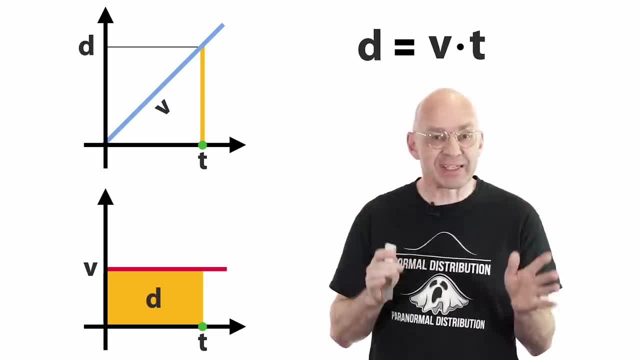 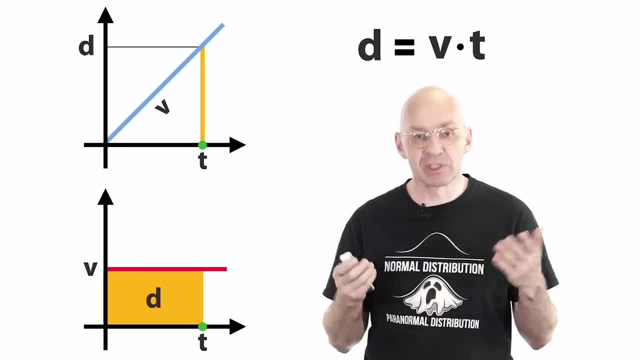 this orange rectangle. Wait what Well? the rectangle is v high and t wide, and so its area is v times t, which is equal to the distance. So what's the answer to our original question? How do you extract the distance traveled above from the speed? 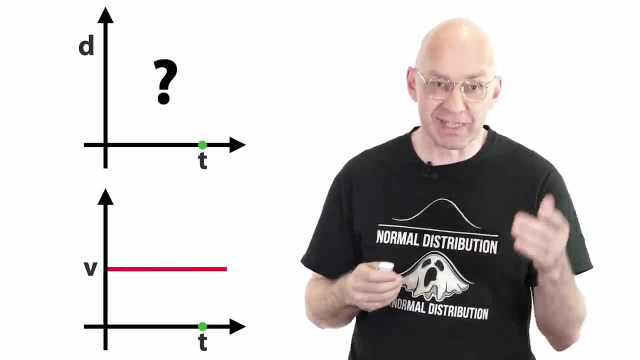 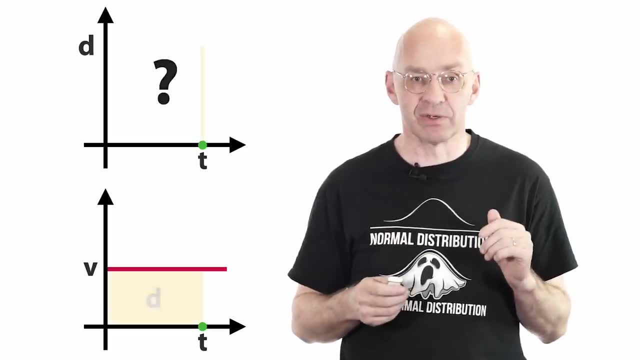 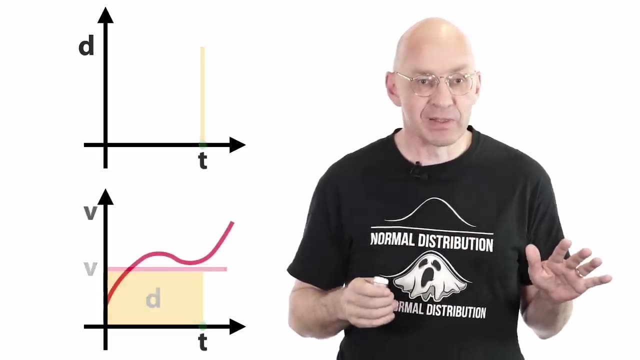 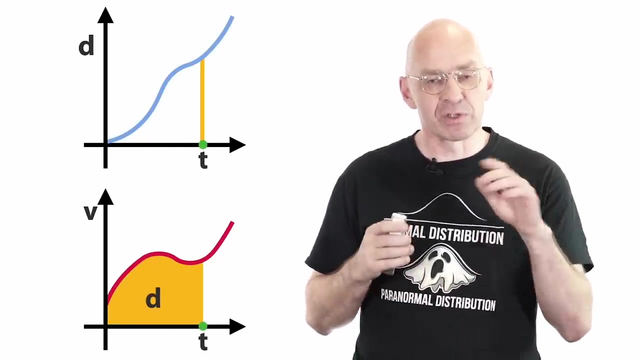 time diagram below. Well, as we've seen in the case of constant speed, the answer is: the distance traveled is simply the area under the curve. Nice, And actually it turns out that this is true in general. Take any speed time diagram, then the distance traveled is just the area under the curve. Very nice, isn't it? And also, 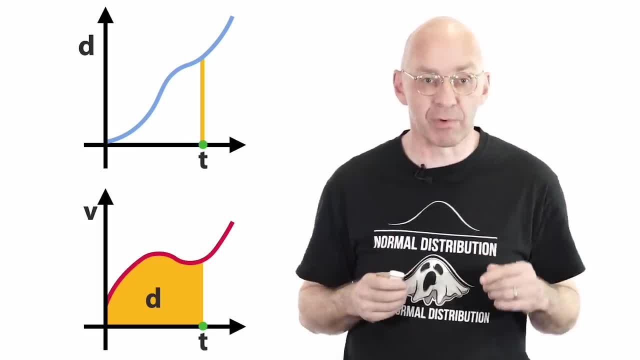 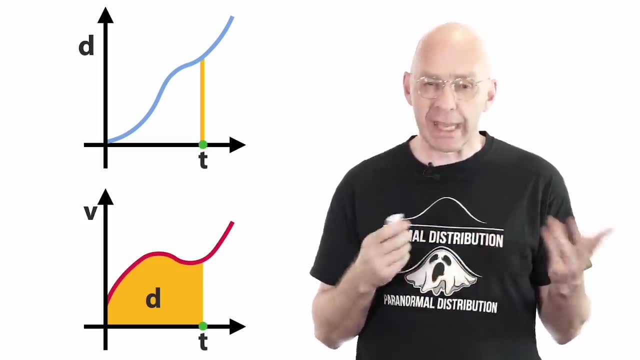 not very hard to see that this is true by approximating things at the bottom with rectangles. Anyway, that's how the speedometer and odometer readings of our car are connected. Okay, Well, what about going the other way? What if we start with the top diagram, the? 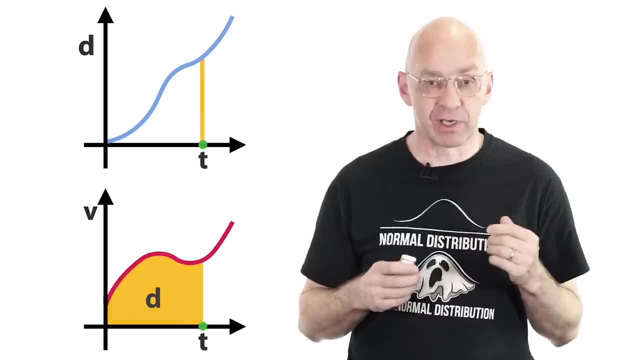 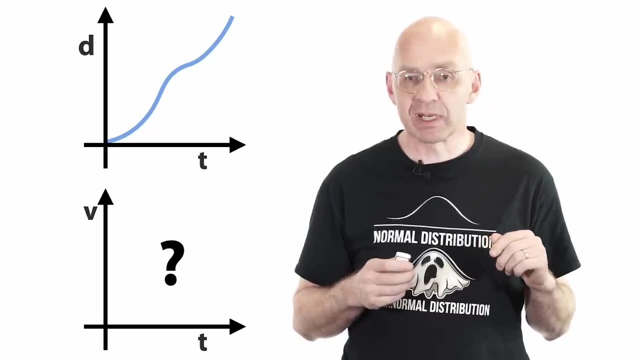 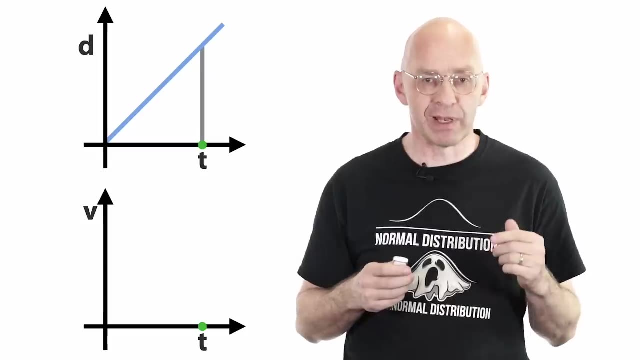 distance time diagram, which corresponds to the odometer reading of your car. How can we reverse engineer the speed time diagram from that? Well, what's the answer? in the simple straight line case that we just considered, As we already said here, the speed at time t is simply the slope of the line, which, of course, is the same. 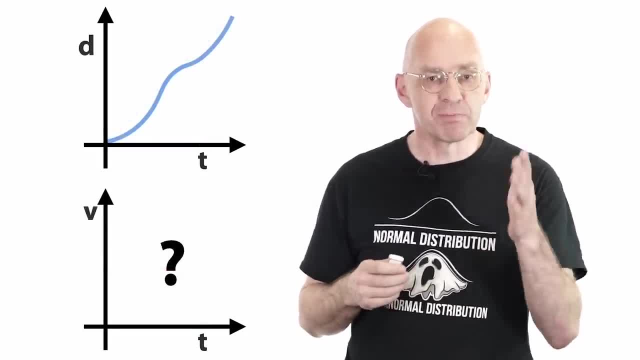 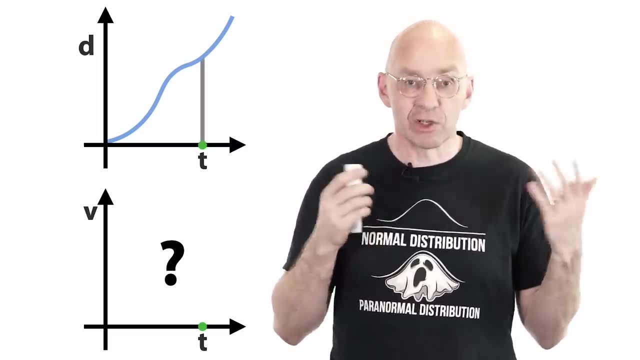 for all t. What about in general? What's the speed at time t? Well, unlike a line, a general curve like this does not have just one slope. It's slope is different at different times. In fact, at time t, the slope of the 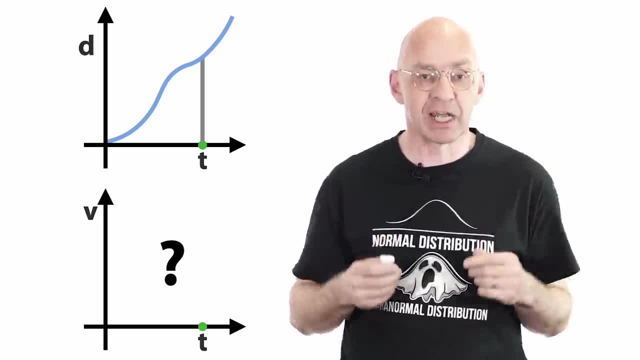 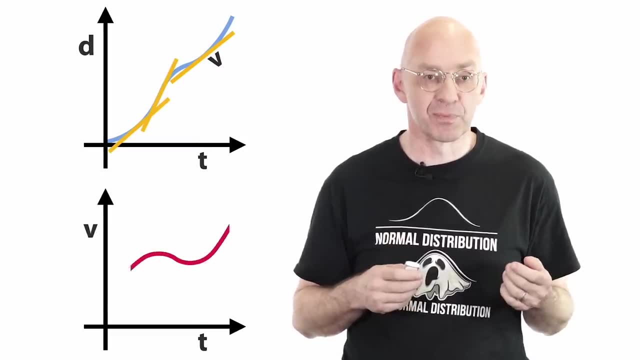 curve is equal to the slope of the tangent line, the line that touches the curve at this point, And of course the slope of the tangent is different at different points. Anyway, to go from top to bottom, we simply calculate the slope. Also neat. 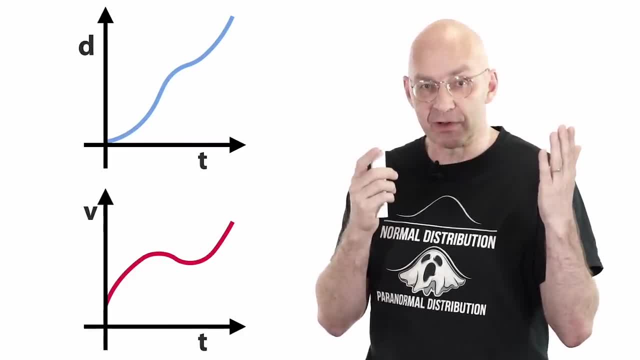 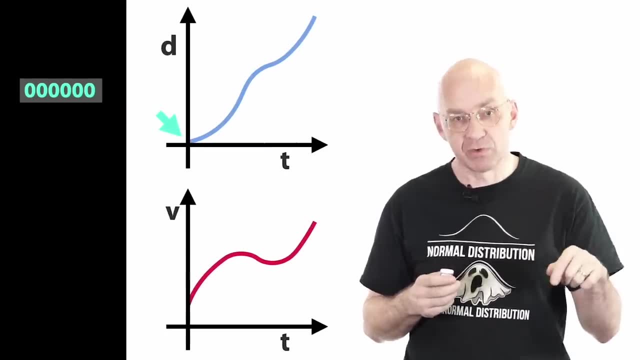 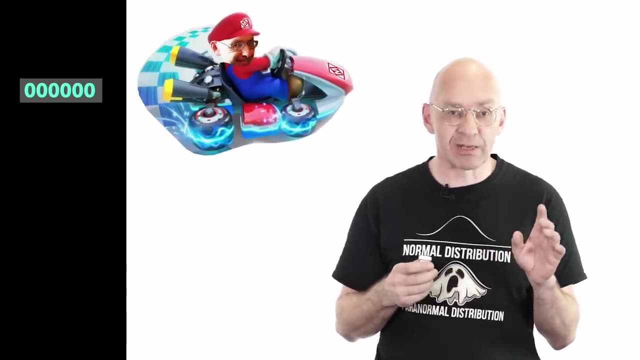 To summarize, the diagram at the top records the odometer reading of my car, with the odometer set to zero when we start recording. On the other hand, diagram at the bottom records the speedometer reading over time. Also, the Mathologer mobile is a vintage sports car with a mechanical odometer which winds. 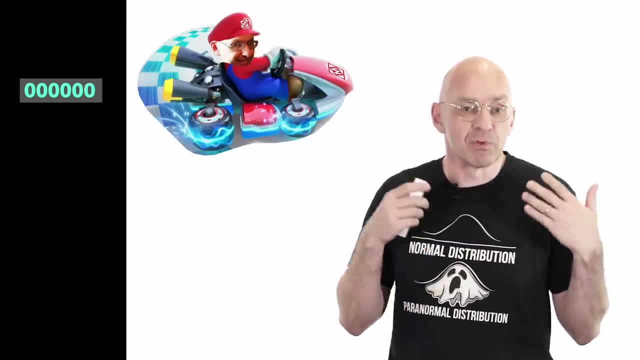 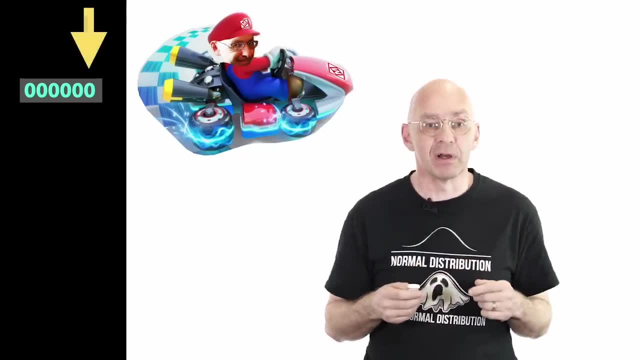 backwards when the car moves in reverse. And if I just move backwards beyond zero- the place where I started recording- I'll record distance as negative distance there. Okay, so we're going forward. so the odometer is going up. now we're going backwards, it's going. 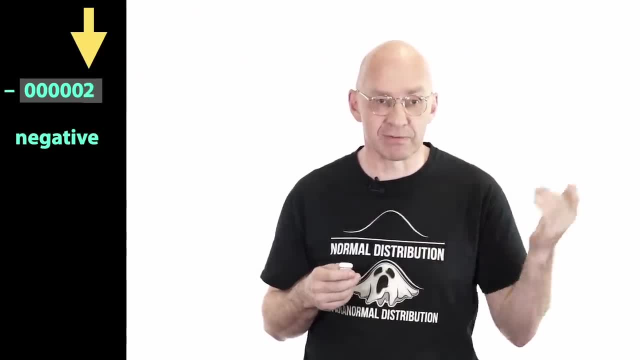 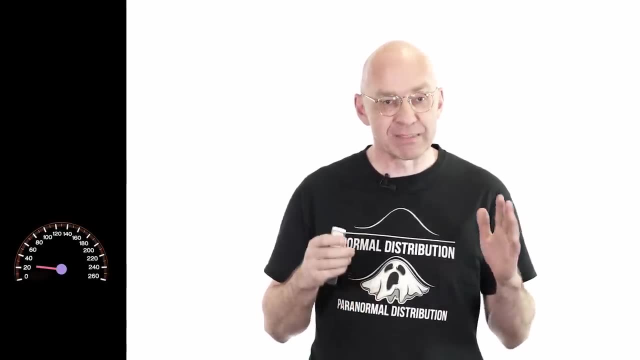 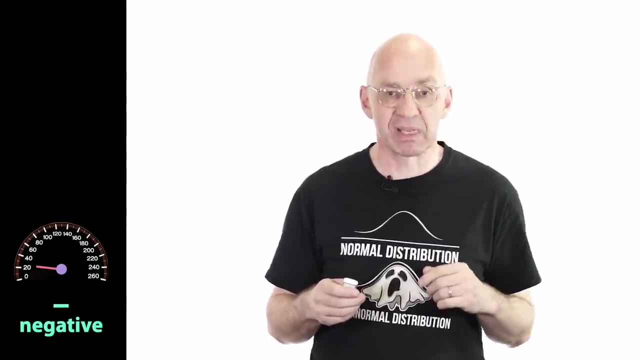 down and beyond the point where we started. it's going to the negative Also. the Mathologer also. when the Mathologer moves in, reverse speed is recorded as a negative number there, something like this: Okay, so car's moving backwards, so negative speed, okay. 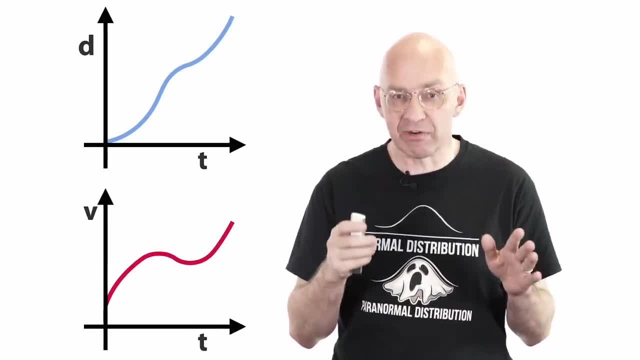 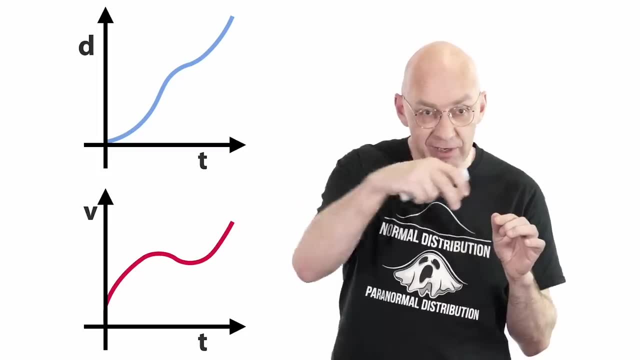 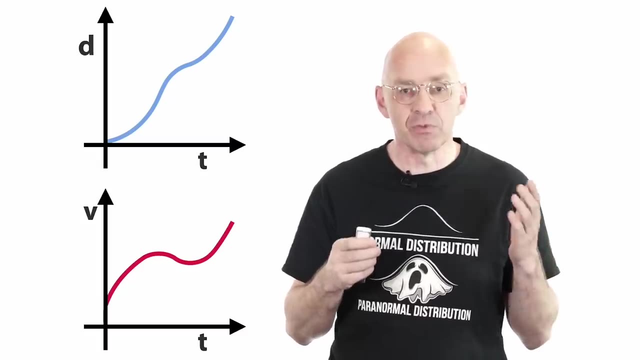 With these recording conventions locked in, I can, at least in theory, create any shape function at the bottom or at the top, by suitably moving my car Neat, And by doing so I can perform some really impressive mathematical feats. To give you an example of one such feat, I could move my car in such a way that the 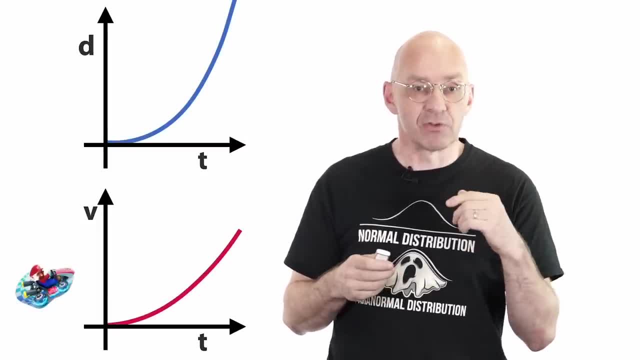 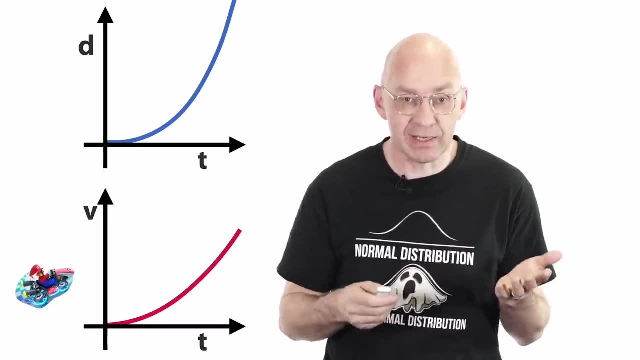 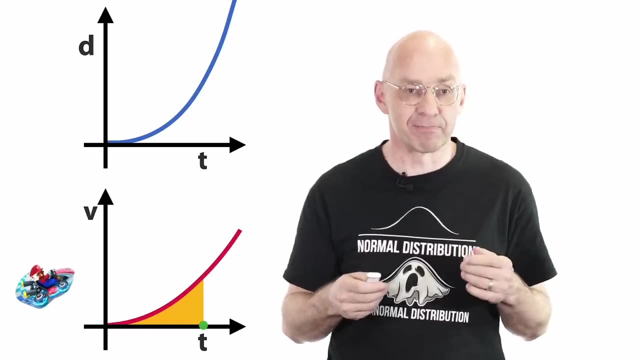 function at the bottom is t squared. There the red curve, that's t squared and the blue curve records the corresponding distance. But then I can calculate the area here under t squared by simply stopping the car at time. t, Then the odometer reading at this point is the area. How amazing is that. 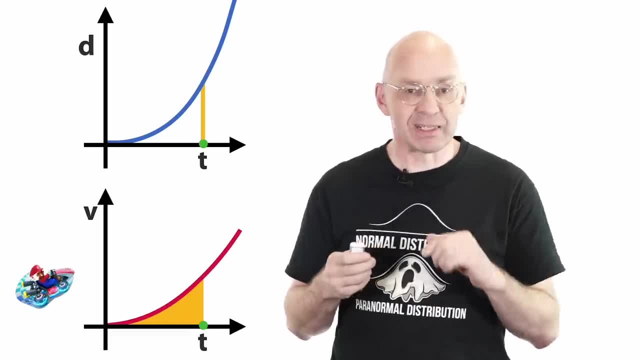 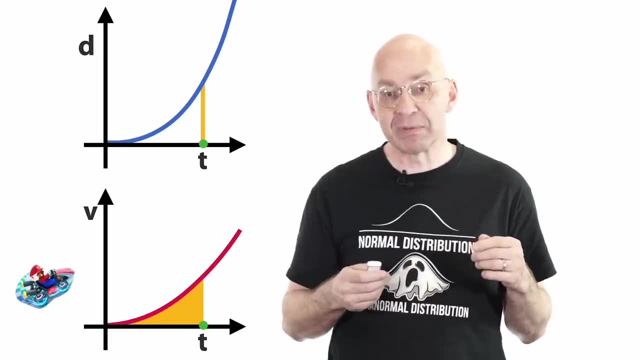 Calculating areas with your car. The first precise calculation of this pretty complicated area under t squared is essentially due to Archimedes and at that point in history amounted to a big discovery. But with our setup we can do much, much, much more than just calculate the area under one curve. In theory, this: 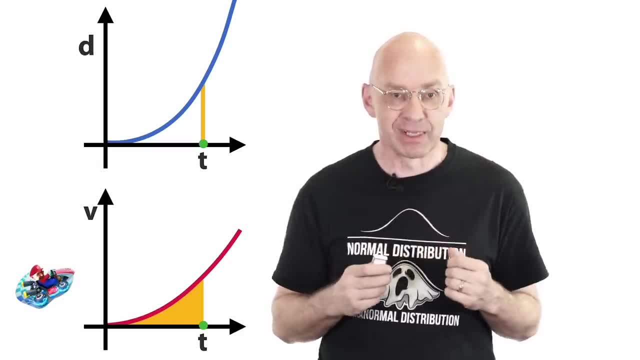 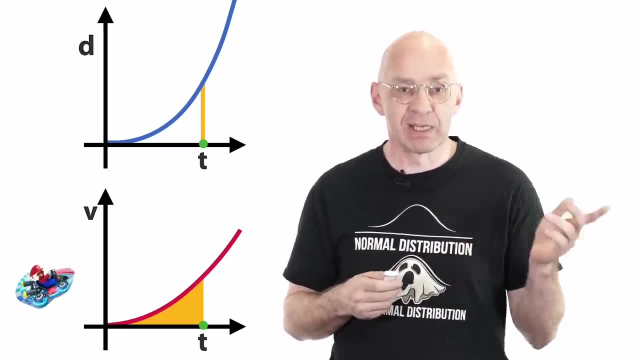 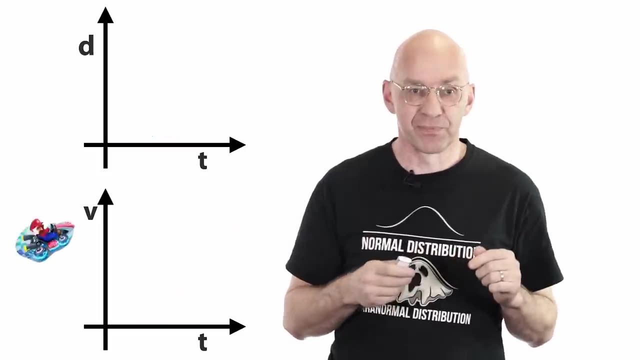 applies to any curve whatsoever- Very powerful. So the things we're playing around with here appear to be useful beyond flipping between speed and distance. Here's another example of a nice application of our game. Let's trace another curve, but this time one at the top Now, when I move my car, so that the 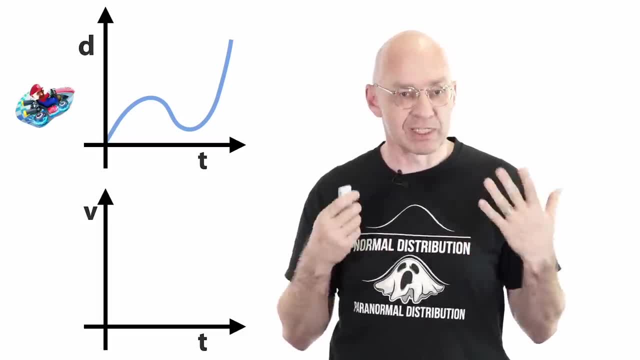 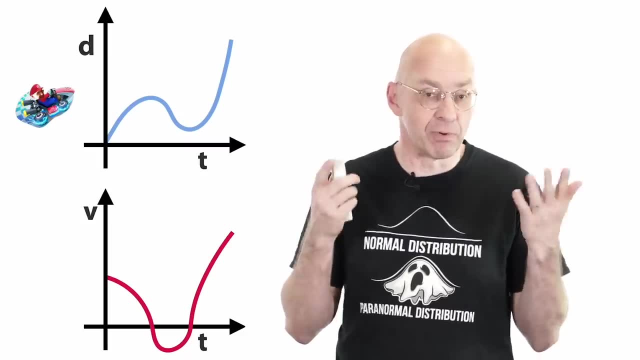 distance traveled is what's shown in this diagram. the corresponding speed diagram below looks like this: The top curve may actually have come from some process for which it's important to identify where exactly the peak and the valley, the maximum and the minimum in the diagram occur. Our setup can simplify. 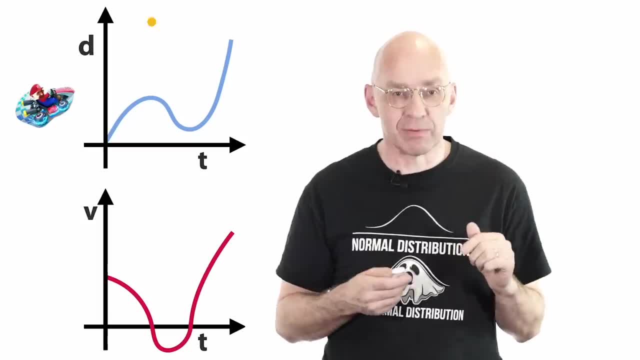 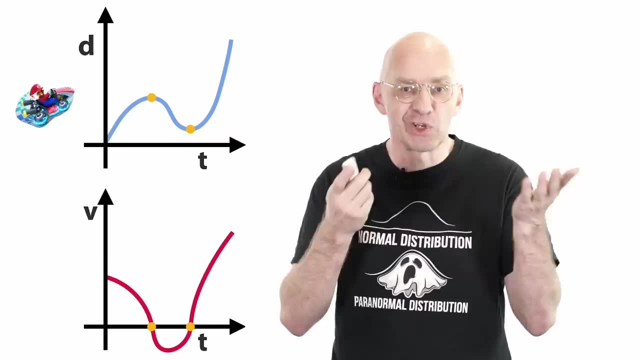 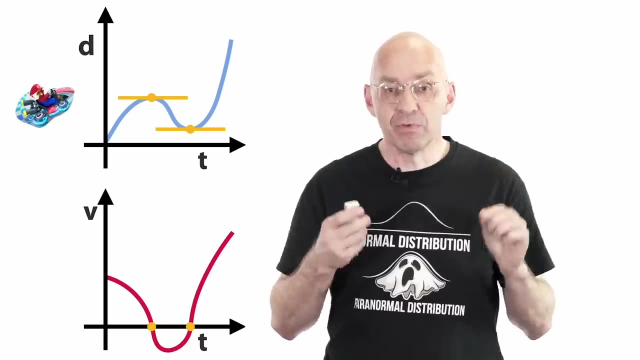 this task. Notice that the peak in the top diagram corresponds to a zero of the function below, Same with the valley. Why is that? Well, because the slopes of the horizontal tangents at these special points are equal to zero. In other words, my car won't be moving at those times. 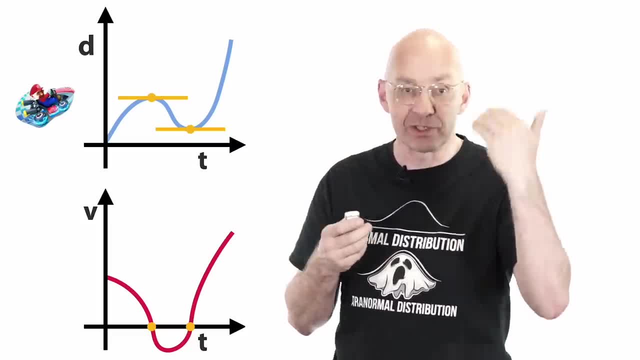 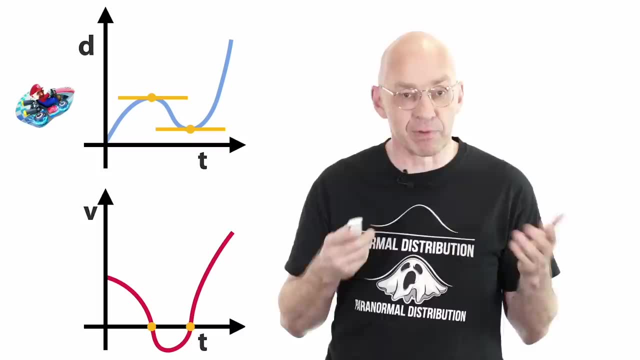 Ok, so translating functions at the top into those at the bottom and using this translation to do things like finding the peaks and valleys of the top curves by simply finding the zeros of the bottom curves, that's called differential calculus, The first terrifying thing that Sylvanus P Thompson 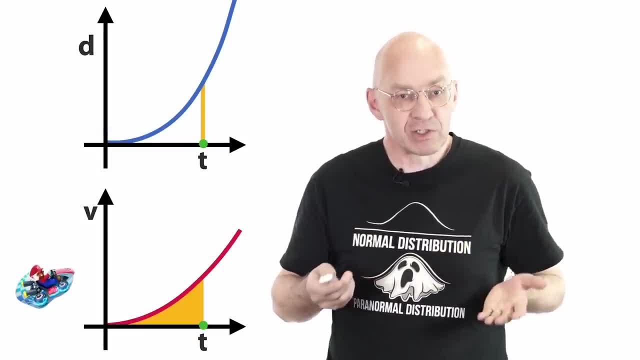 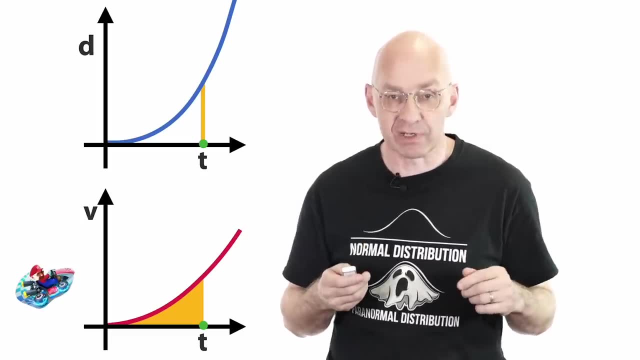 mentioned on the cover of his book, Translating functions at the bottom into those at the top and using this translation to do things like finding areas under the bottom curve. that's called integral calculus, the second terrifying thing, And our kindergarten formula up there nicely captures how 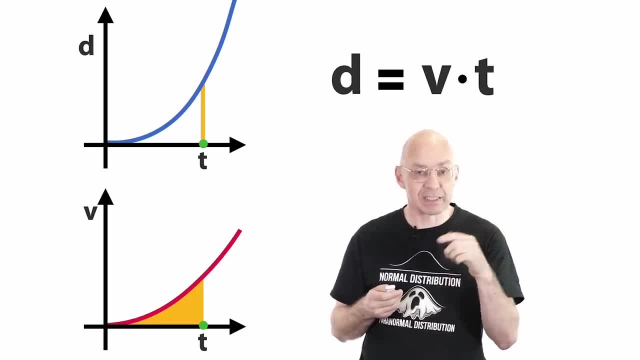 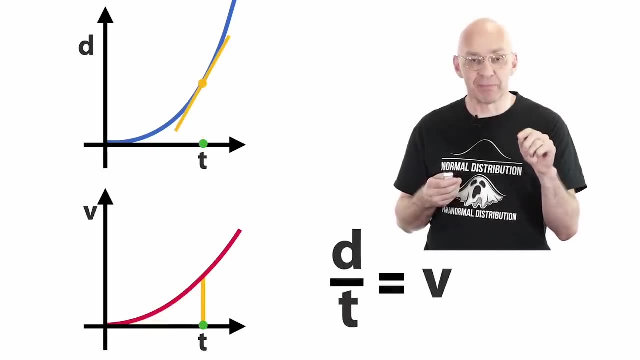 exactly we translate between the top and the bottom, between the distance and the speed. right, Distance equals speed times time, One thing times another. That's area. Our distance is the area under our speed curve. On the other hand, speed equals distance divided by time. One thing divided by another. 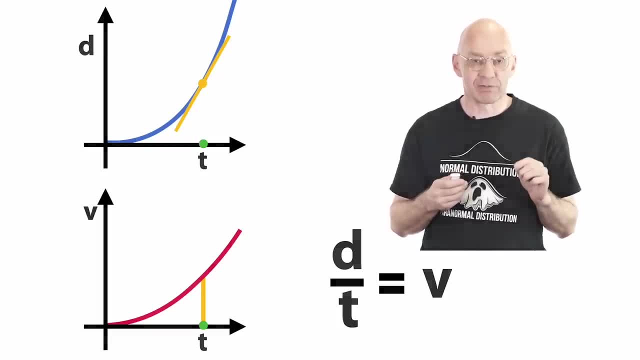 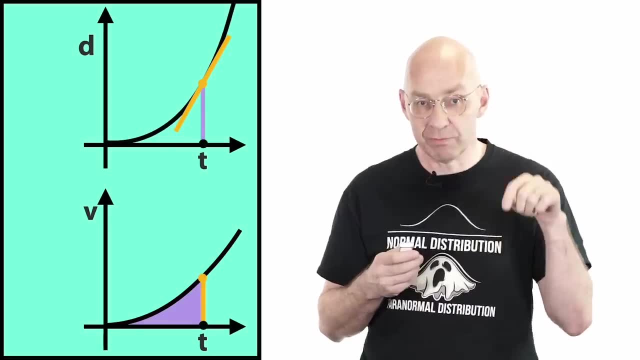 That's slope. Our speed is the slope of our distance graph. Again, distance is the area under the speed graph. Speed is the slope of the distance graph: Top to bottom slope, Bottom to top area, Top to bottom slope, Bottom to top area, and so on Burn. 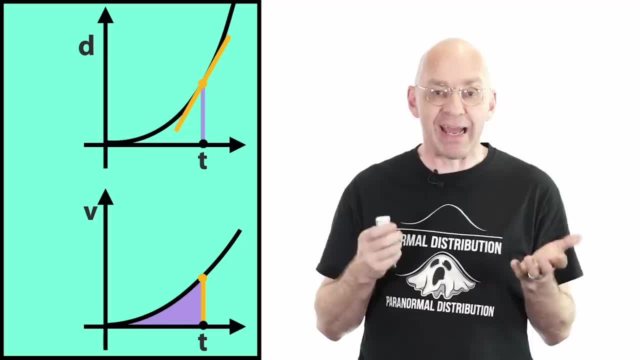 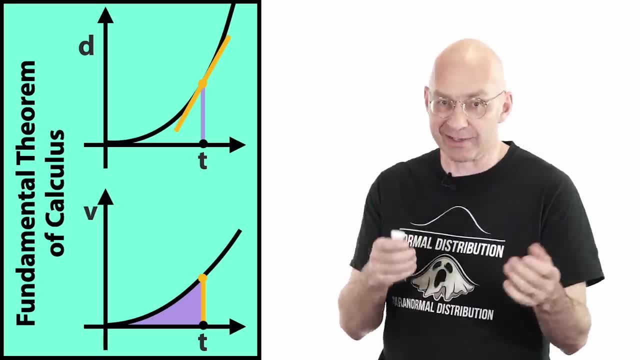 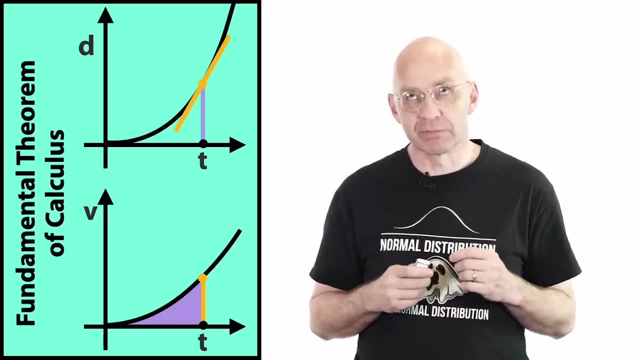 this into your memory. This amazing relationship goes by the grand name of the fundamental theorem of calculus. Fundamental as in the most important thing in calculus, The soul of calculus, And it really is. If you followed everything so far, you're now entitled to say: I know calculus Well, sort of Anyway. 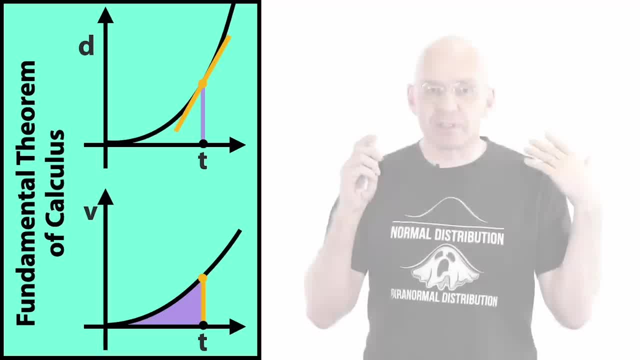 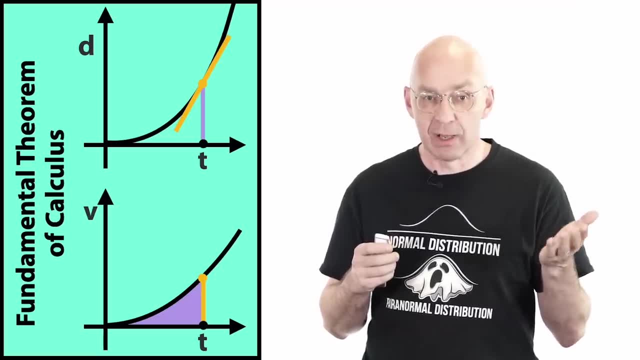 none of what I said so far was terribly terrifying, was it? But of course there's a bit more to calculus. In particular, for all of this to be really useful, we need to be able to perform those translations, preferably without having to worry about speed limits, traffic lights and 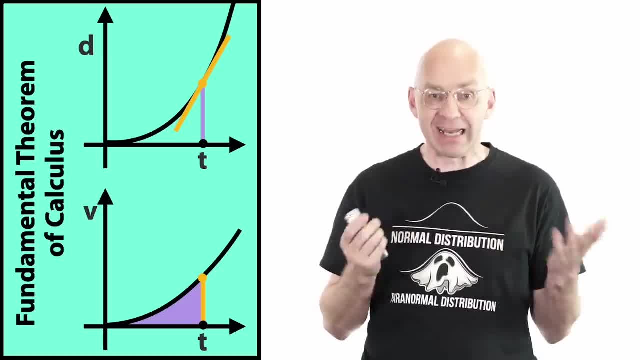 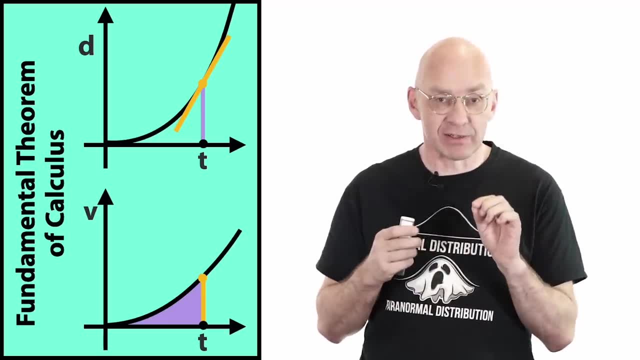 idiot drivers Right, If the functional top is sine, what's the one at the bottom? How can we figure that out? Well, it turns out that differential calculus to go from top to bottom is really super easy and pretty for a vast assortment of 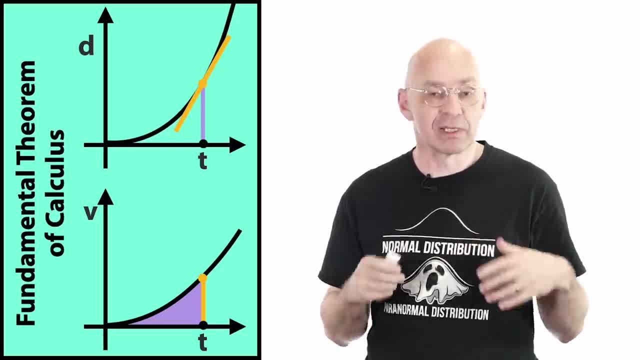 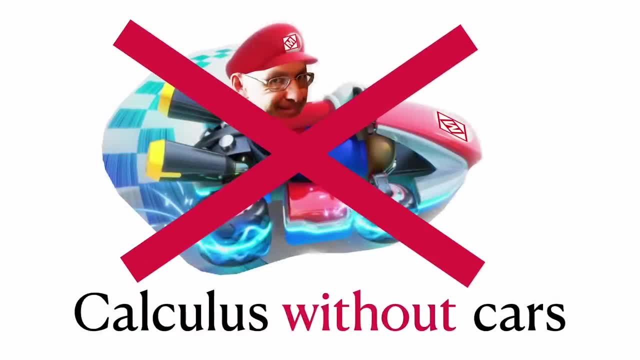 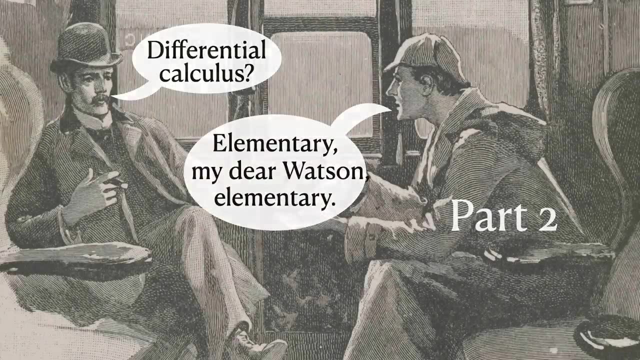 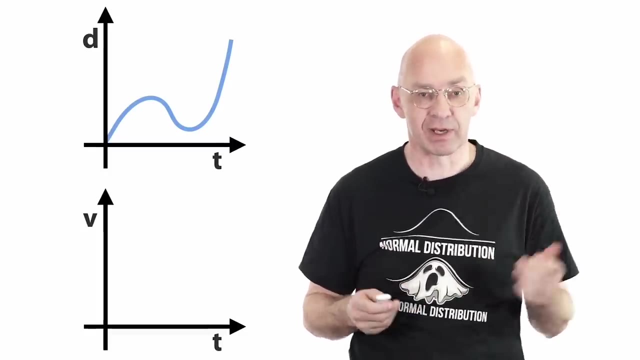 functions. This includes all our favorite functions like the powers, the exponential function, the trigonometric functions and so on. Well, let's have a close look. Okay, let's get away from cars and label the x's at the top and bottom x and y. So 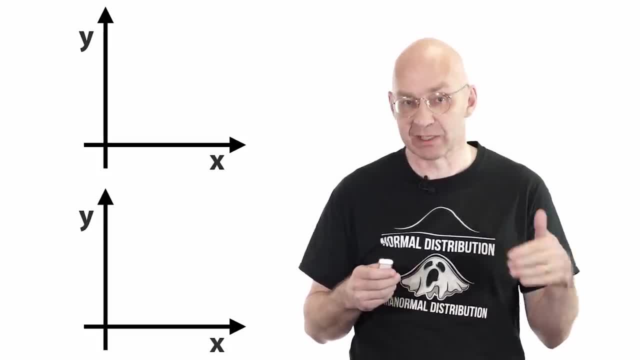 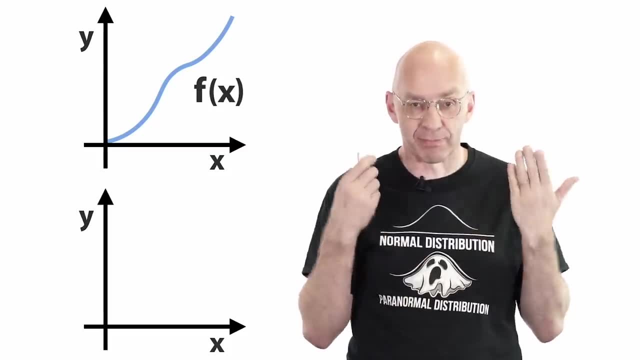 all the functions we'll be talking about are in the variable x, as it's usually the case in school. Second, starting with a function f at the top, the corresponding function at the bottom is called the derivative of f, or f prime As well. 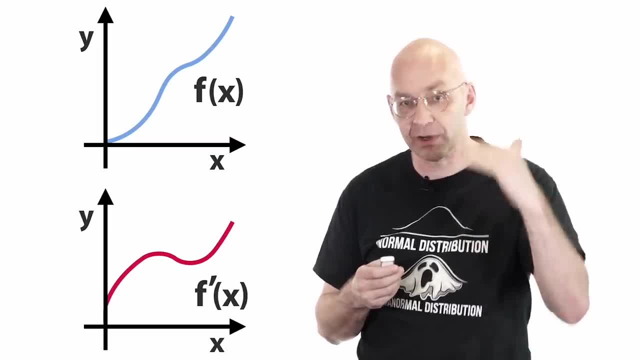 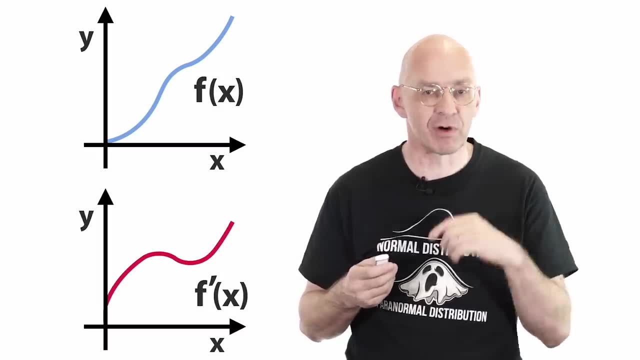 the process of translating the function on top into the one at the bottom is called differentiating. Remember differential calculus. Now let's start by making the function f one of our favorite functions. There f might be a constant function, or x to some power, or one of the trigonometric functions. and 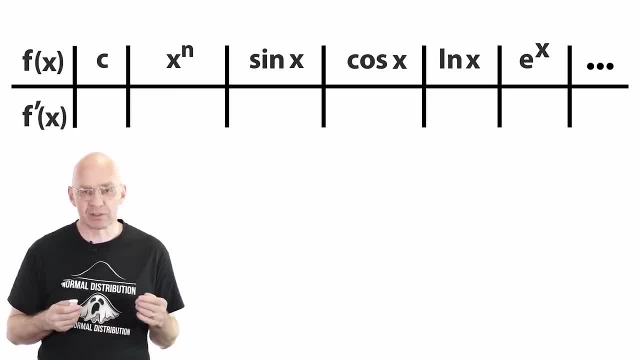 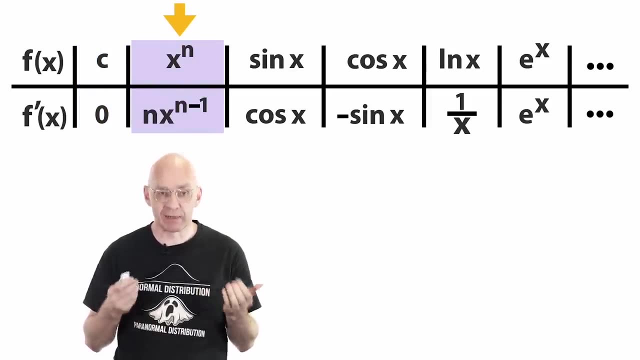 so on. What are the derivatives of those functions? Well, here you go There. the derivative of a constant function, that is its slope, is zero. obviously. The derivative of some power of x is basically x to one less that power Neat. 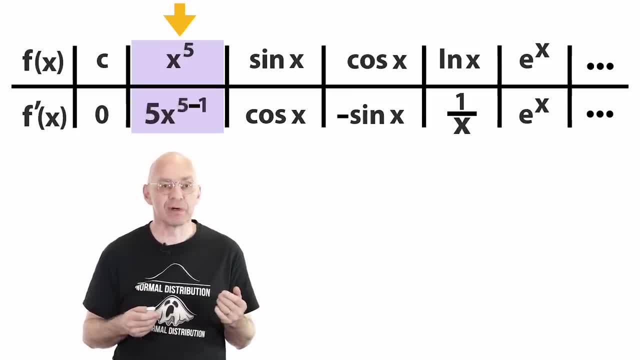 huh. For example, for n is equal to five. we get this Okay there. the derivative of x to the power of five is five times x to the power of four, Five, four, so one less. The derivative of sine turns out to be cosine and the derivative of cosine is: 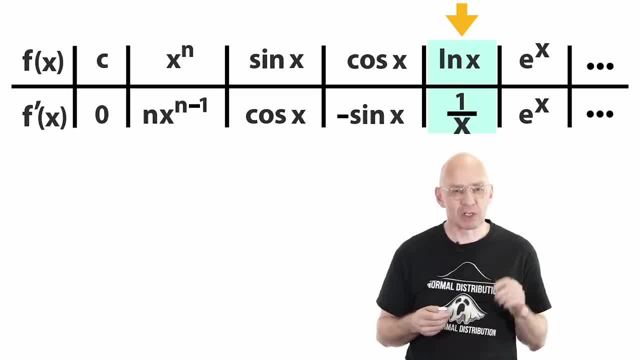 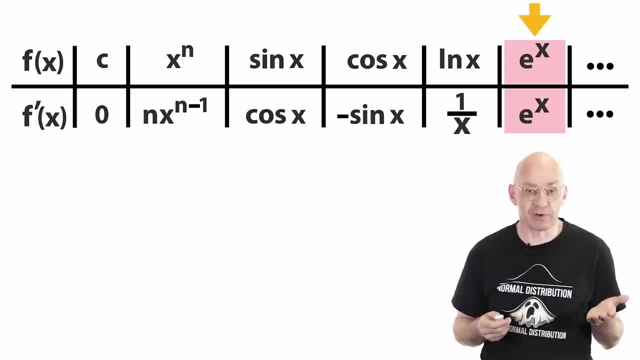 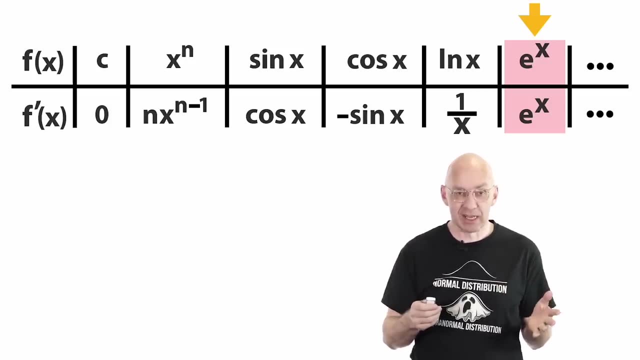 minus sine. Very pretty. Here's something quite surprising. The complicated natural logarithm function has the simple one over x as its derivative. The exponential function is its own derivative- also super nifty. And, as I said, we'll actually derive all these derivatives as part of the animation at. 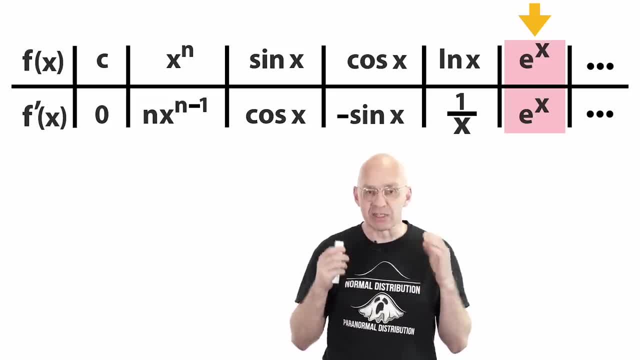 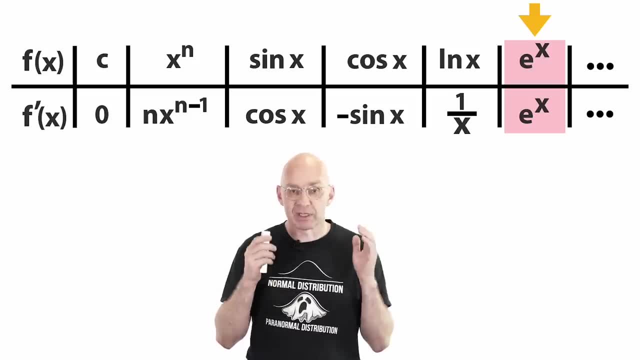 the end of the video. Important observation here is that essentially all functions in our list have derivatives that also occur at the top of our list, with a constant factor thrown in the mix, perhaps right. We mostly see the same stuff at the top and at the bottom. Great Next, starting with the functions in our 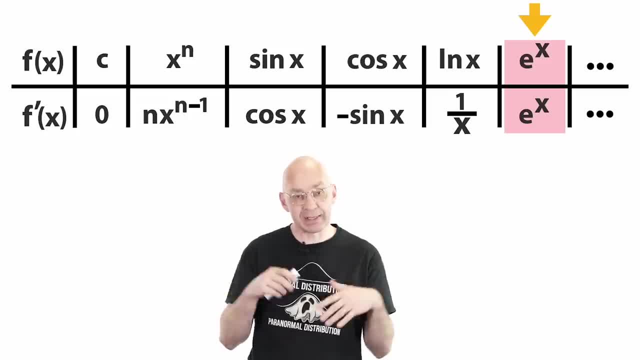 list. we can build lots and lots of more complicated functions by adding, subtracting, multiplying and dividing and substituting one function into another. Well, of course, in calculus there are many other important, more complicated ways to make up new functions from old ones, For example by constructing the inverse of functions. But let's not worry. 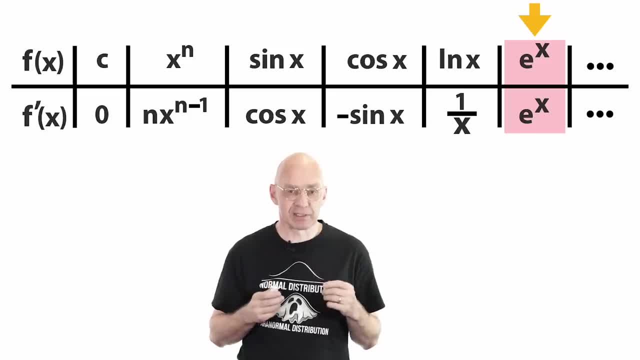 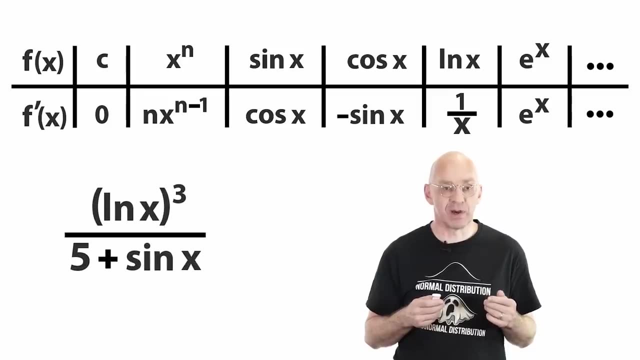 about any of those other ways for the moment and stick with the basics To make new functions from old ones. for starters, we'll only add, subtract, multiply, divide and substitute. Cool, Here's an example. Okay, so add those two together, put one into the other and divide Those basic atom functions. 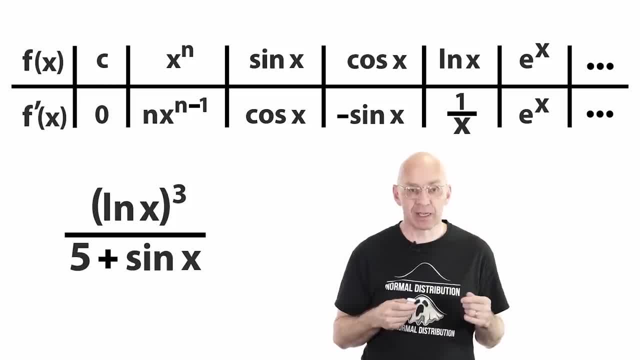 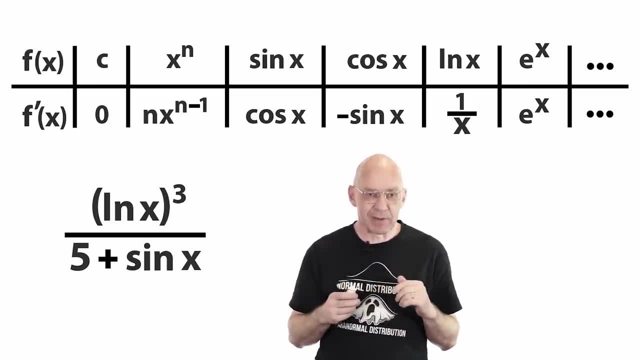 up there, plus the complicated functions that can be constructed like this from them are called the elementary functions. Yeah, I know that thing over there doesn't really look very elementary, but it's really elementary in the sense that it's built from our atom functions, using only those five elementary ways of combining functions. Now, one of the 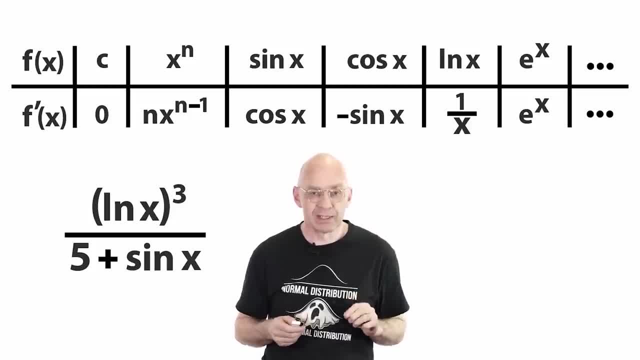 main reasons why calculus is so incredibly beautiful and useful is that the derivative of every elementary function is also an elementary function Plus. and that's really the killer. it's not hard at all to find these derivatives, Not harder than basic algebra. You can teach a monkey. 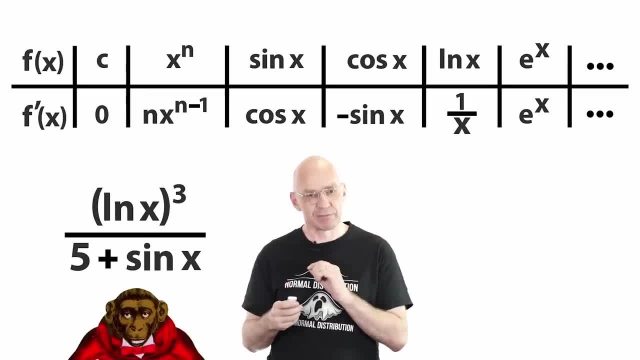 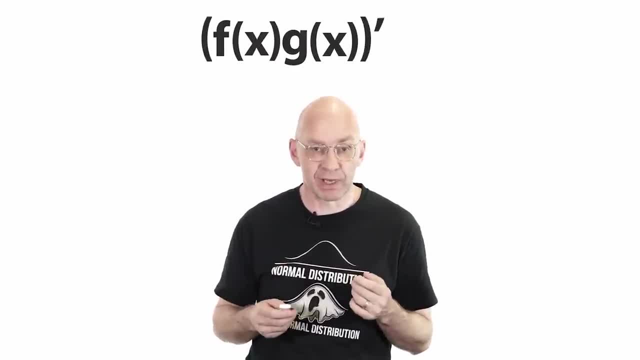 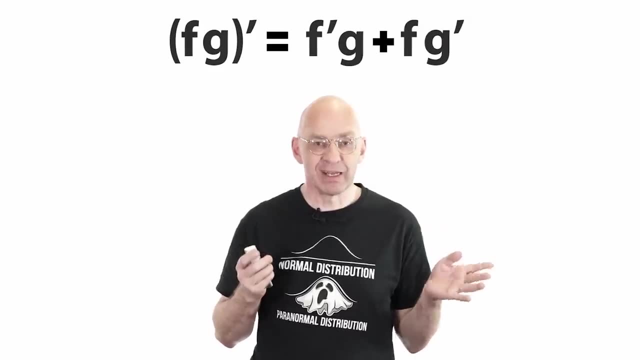 to find the derivative of an elementary function. Why is that? Well, let's say you multiply two functions. I'll show you in the animation at the end that the derivative of this product is this: Quite nice, A bit messy, so let's simplify it a bit. Ah, much nicer. Anyway, the two functions f and 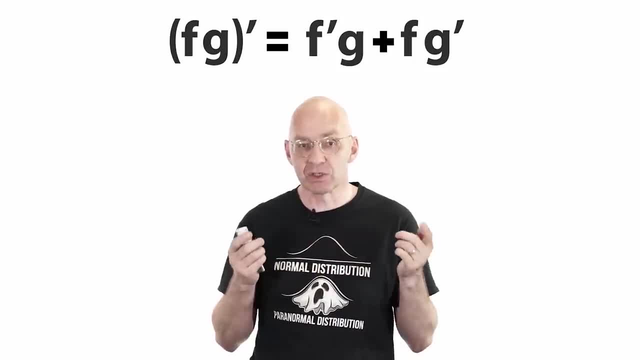 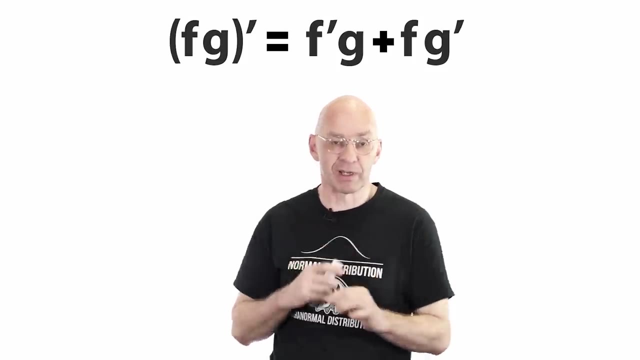 g and the derivatives f prime and g prime are combined using two of our basic operations: plus and times. Okay, And so if these four functions are all elementary, then the semi-productive combination of these four elementary functions on the right side is also elementary, right? 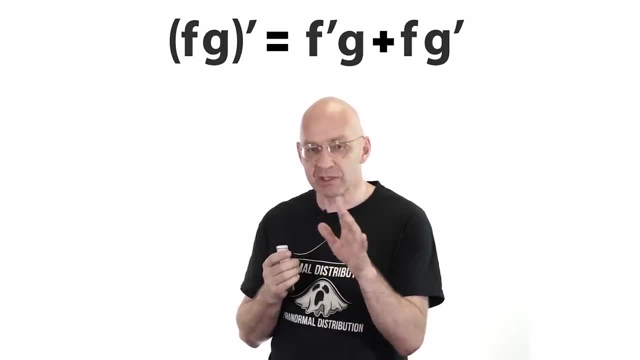 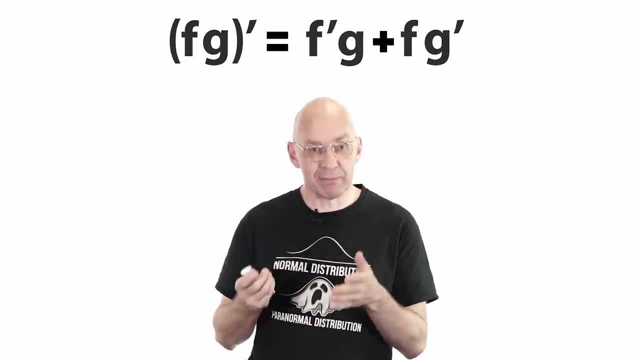 Again, if f and g and the derivatives are elementary, then the derivative of the product f times g is also elementary, elementary. Okay, the same is true for the derivatives of the sum, the difference and quotient of two functions and for the derivative of the substitution of. 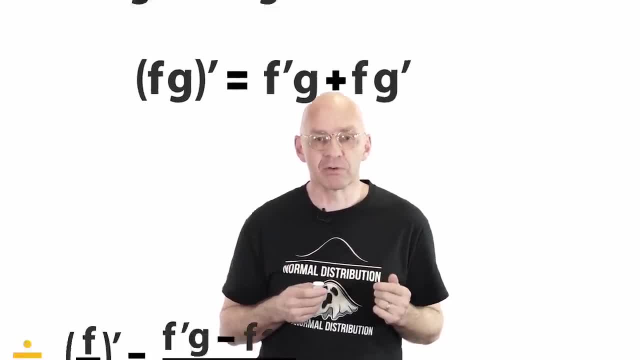 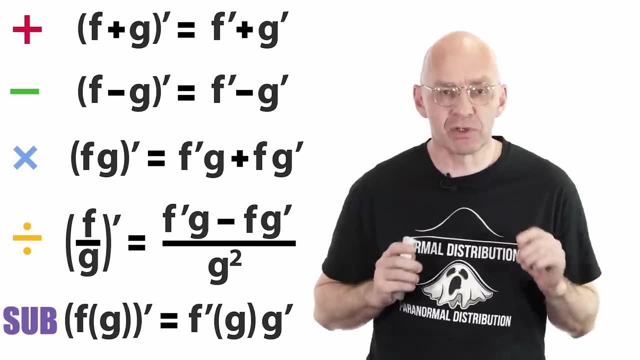 one function into another. Here are the corresponding formulas or rules. All pretty simple There: plus, minus, divided. one function subtracted another. Okay, now let me show you how all this translates into an elementary function, having an elementary derivative, and how to find this. 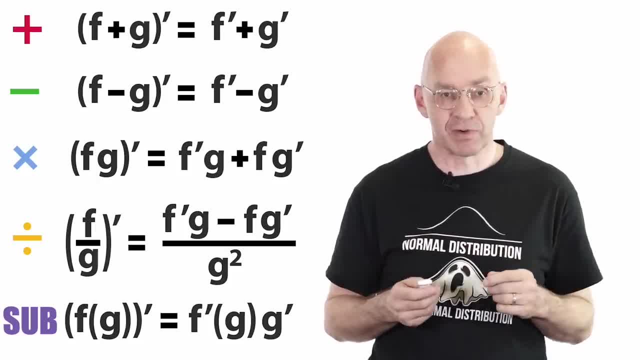 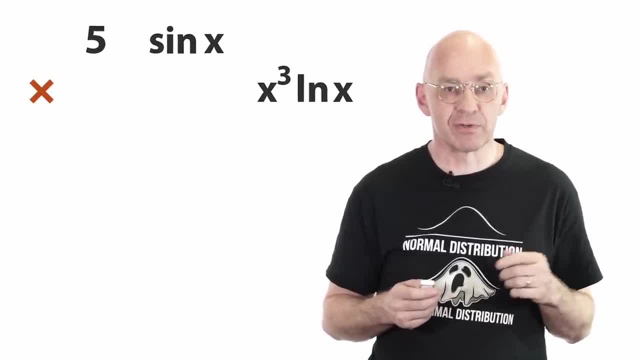 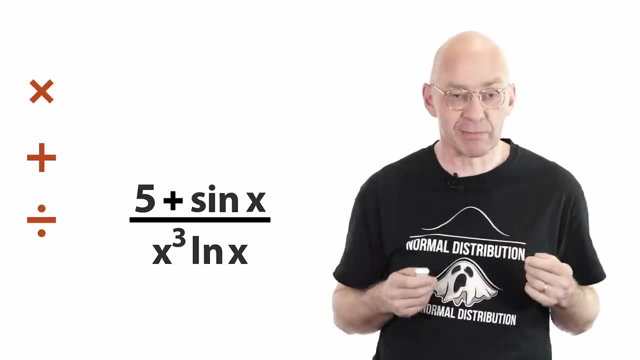 derivative. For this, let's make up another elementary function from these four atoms. First we multiply the last two functions together, then we add the first two and finally we divide the function on the left by the function on the right. So we use three operations to make this elementary function. First, 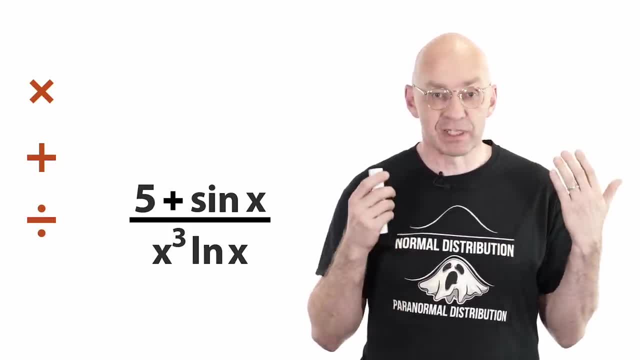 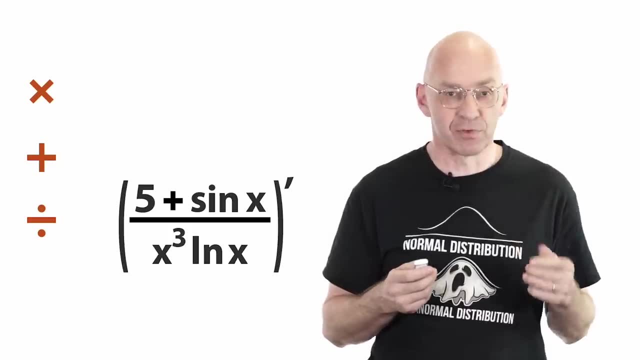 multiplication, then an addition and a division. Now we want to find the derivative of this function. For this we'll use the rules that correspond to these three operations in reverse order. So first the quotient rule, then the sum rule and finally the product rule. And as we're doing this, 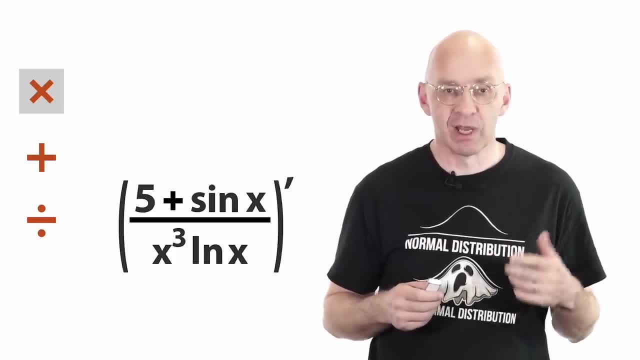 we'll also feed in the derivatives of the four atoms we started with whenever we come across them, And once the last atom has been processed, we'll be finished, Really completely automatic. Pour yourself a cup of chocolate and enjoy the algebra, autopilot and the funky music. 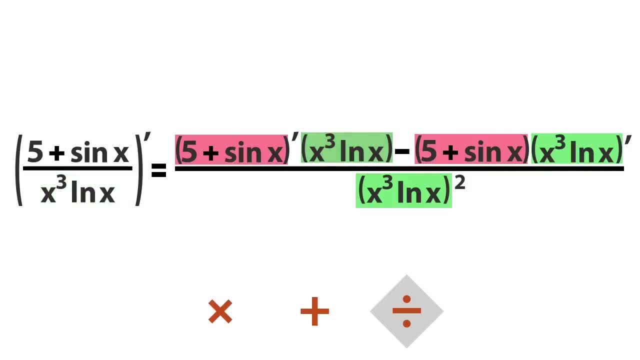 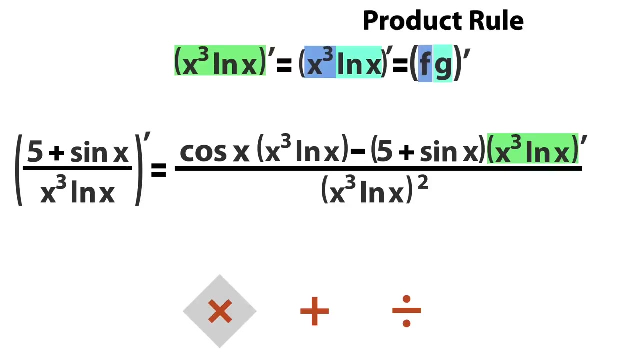 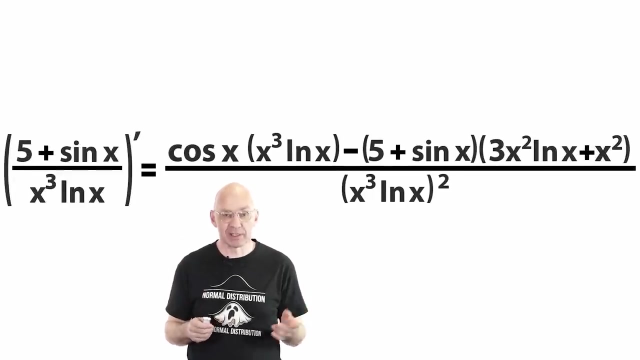 Thank you for watching this video. I hope you enjoyed it and I'll see you in the next one. Thank you for watching this video. I hope you enjoyed it and I'll see you in the next one. But- and that's important- you really just have to follow your nose to get to it. 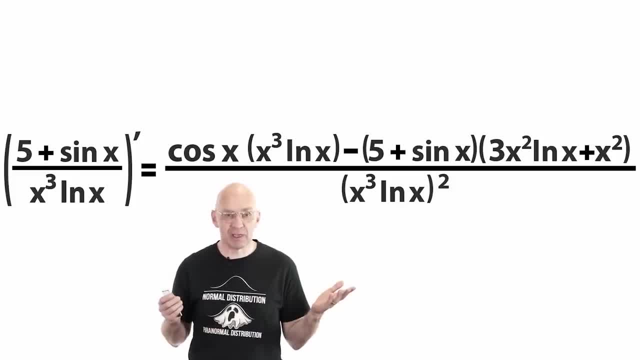 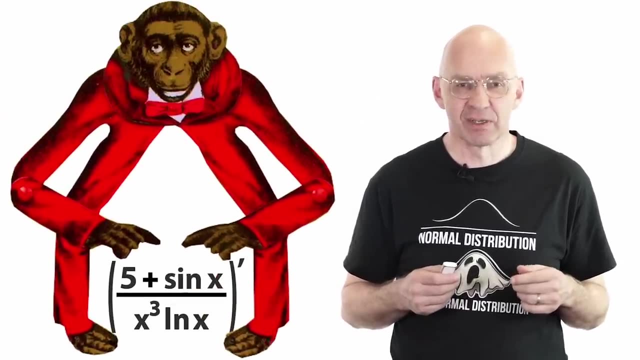 Completely automatic. So we start with an elementary function and by applying our rules, which only involve elementary operations, we generate a sequence of elementary expressions culminating in the elementary derivative. As I said, you can teach a monkey to do differential calculus. Remember what all this is good for? 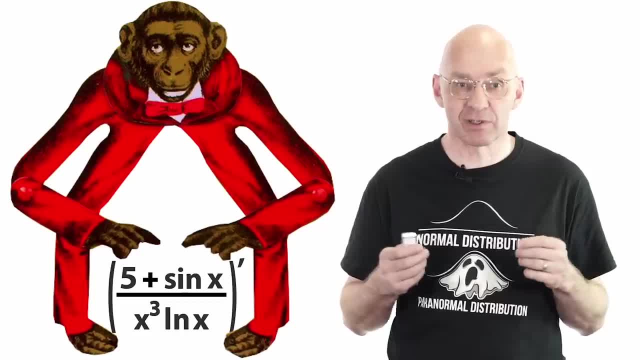 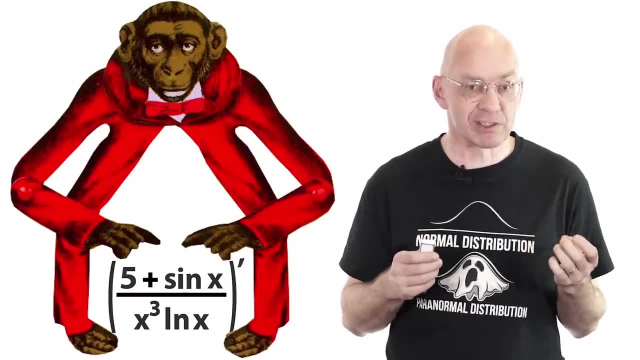 Differentiating distance as a function of time gives speed as a function of time. Differentiate again, you get L-acceleration. If you are faced with a ferocious function in the wild, you can reduce the task of finding the maxima and minima of the function to finding the zeros of the. 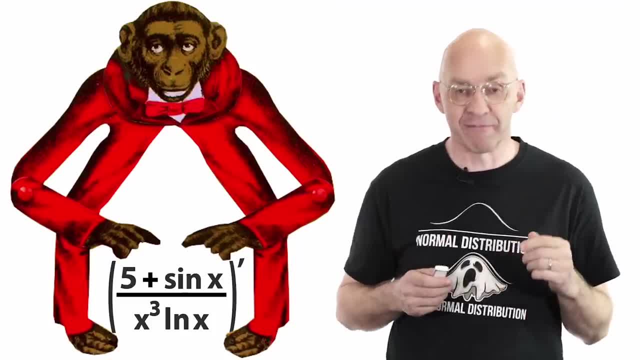 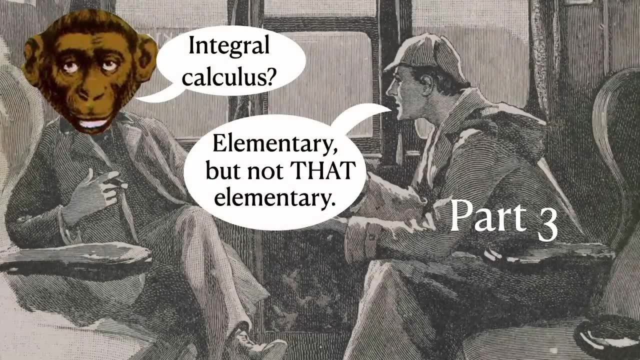 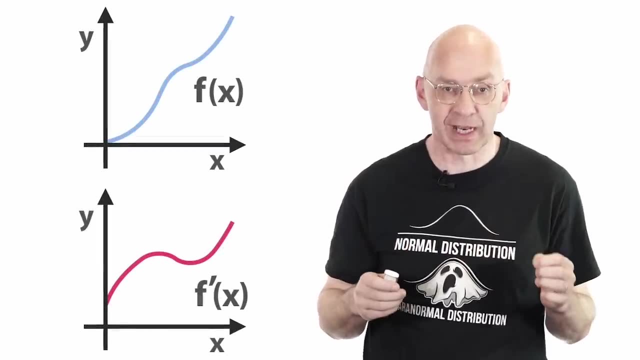 derivative and much, much, much more Very useful and very powerful stuff. Okay, so once I've actually proved to you that the derivatives of our atoms and those rules for finding derivatives are what I claimed they are, then I'll show you how to do it. 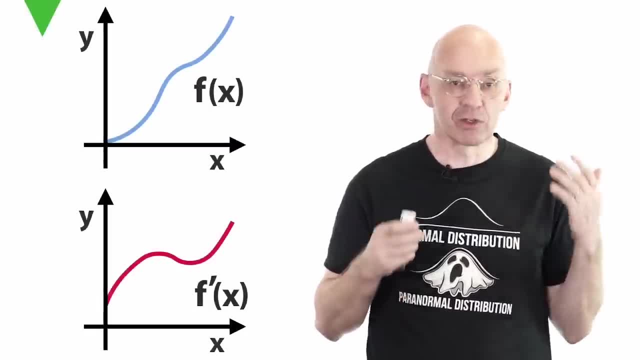 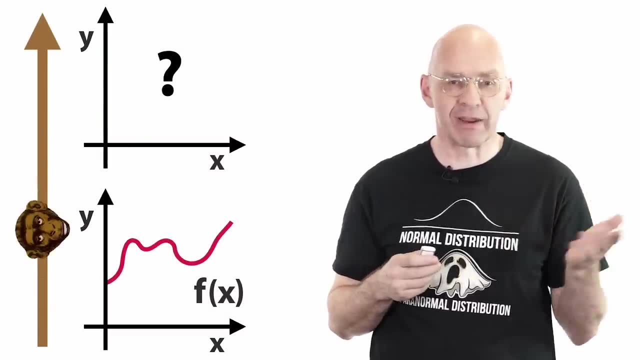 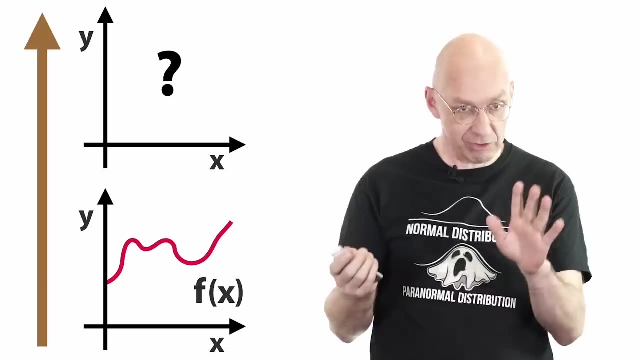 Then differential calculus to go from the top to the bottom looks pretty much under control. How about integral calculus, going from bottom to top? All that cute area-finding business? Well, using our fundamental theorem of calculus, you partly get this for free. What? How? Well, let's say the function at the bottom is. 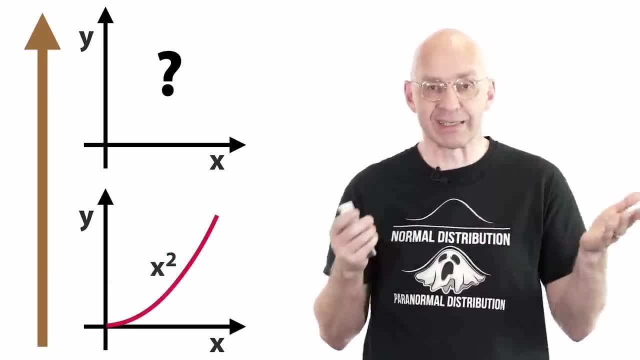 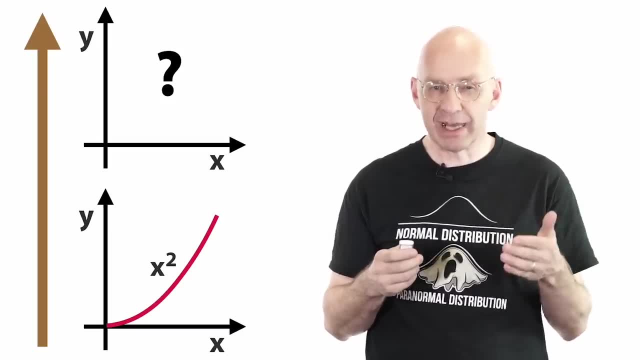 really x squared. What's the function at the top? Well easy, We just have to find the antiderivative of x squared, that is, the function whose derivative is x squared. For that, let's have a look at the list of derivatives of our basic building. 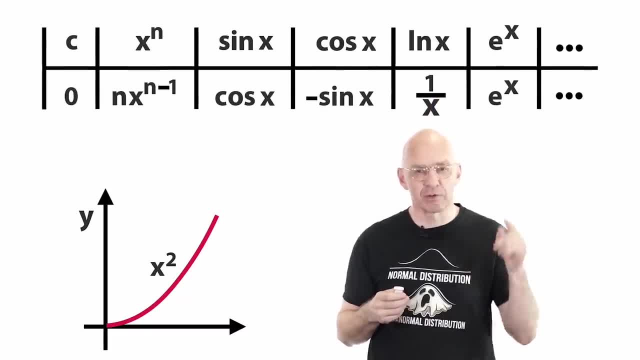 blocks. Maybe we get lucky. We've been reading this list from top to bottom, but of course we can also read it from bottom to top, right. So is there an x squared among the entries at the bottom? Well, yes, right there. If we choose, n is. 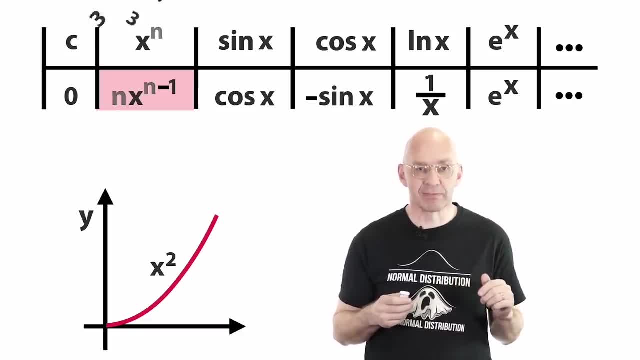 equal to 3, we get x squared in the red There, 3x squared- Almost what we want. Well, to get x squared, just divide by 3, both at the top and at the bottom. Yes, don't worry, we can do that. Okay, so the antiderivative of x squared is 1. third, 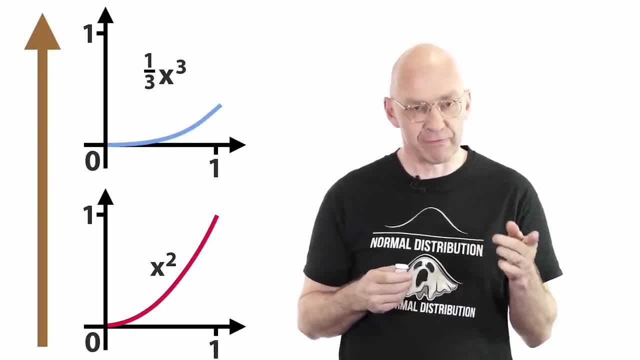 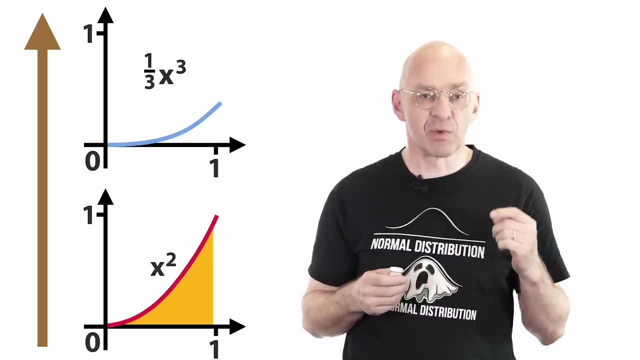 x cubed. And so if, for example, we're interested in the area under x squared between 0 and 1, that area is just 1 third x cubed evaluated at 1.. So 1 third times 1 cube, that's. 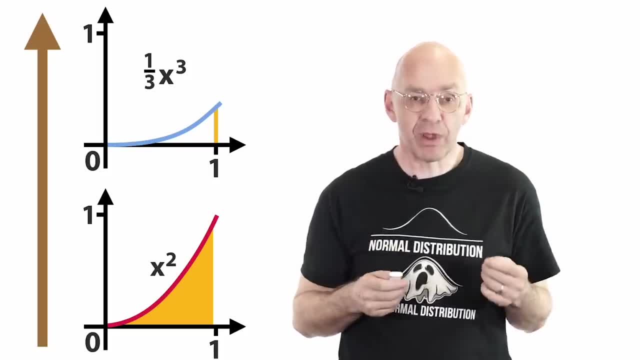 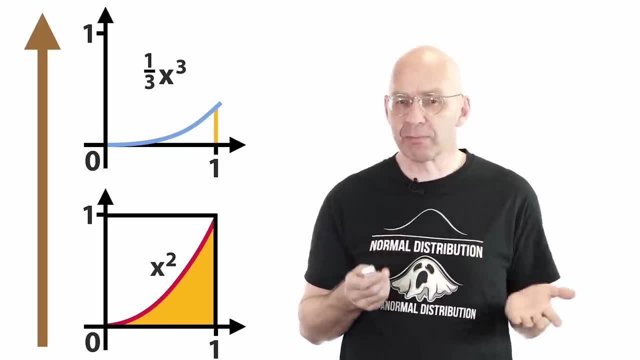 just 1 third. In other words, this area is just 1 third the area of this, 1 times 1 square. Super pretty And also pretty surprising. the first time you see this. Why would such a complicated area have such a simple value of an area? Anyway, important. 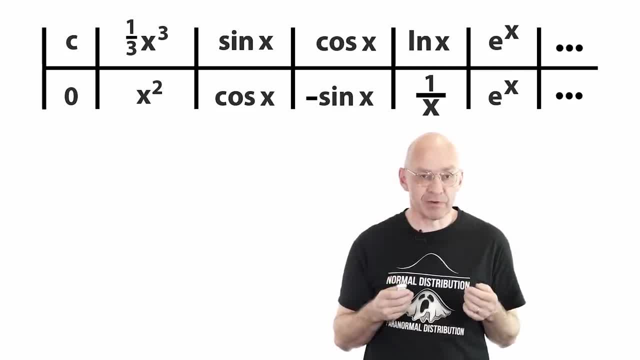 insight. reading from bottom up, our table of derivatives immediately gives us the antiderivatives of many key functions for free. That's really nice, isn't it, And super useful. But did you notice one or two little bumps in the road? No, These. 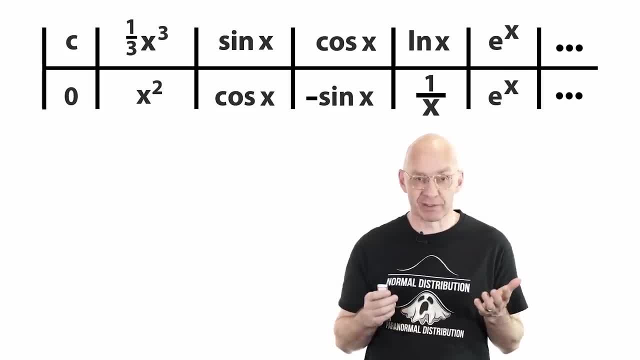 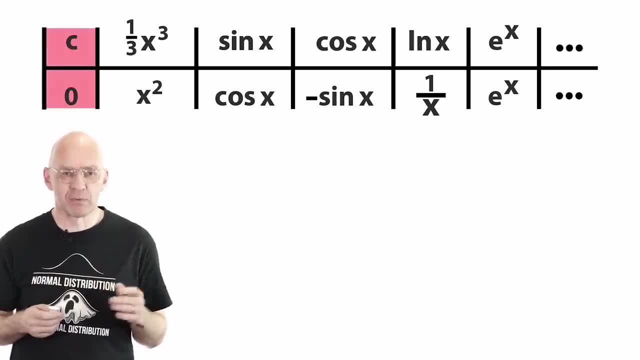 are really minor bumps, But, at the same time, very important ones to smooth out. So let's do that now. What's the bump number one? Well, let's look at the first entry of our list. What's bumpy about that, Can you see? 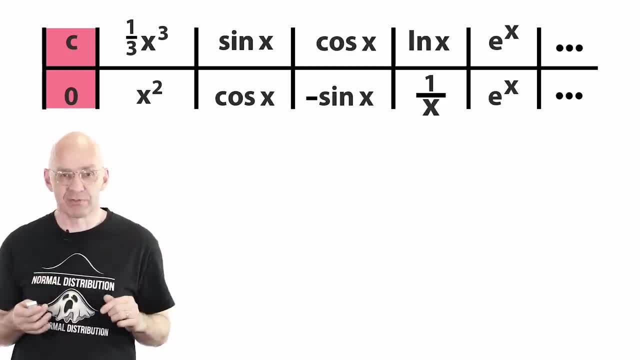 it. Well, the derivative of any constant function is 0, but this means that every constant function is an antiderivative of the zero constant function. Zero does not have just one antiderivative, it's got infinitely many. In fact, just like the zero constant function has these infinitely many antiderivatives, so does 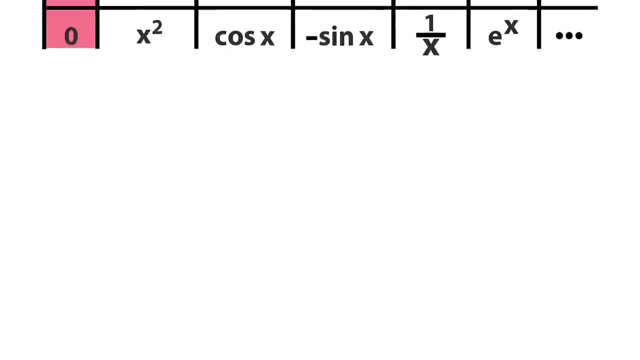 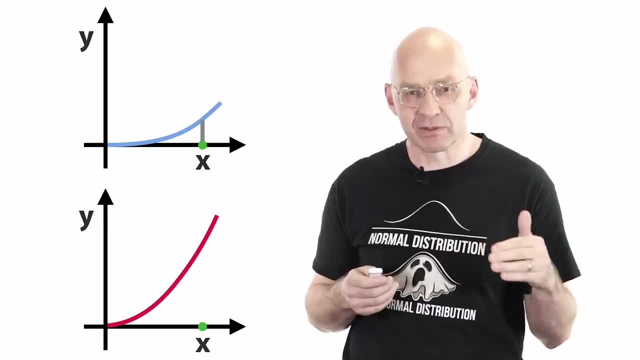 every function. That's actually pretty obvious when you think about it. There, The blue function is an antiderivative of the red function. Again, what this means is that for all x values, the slope at the top is equal to the value at the. 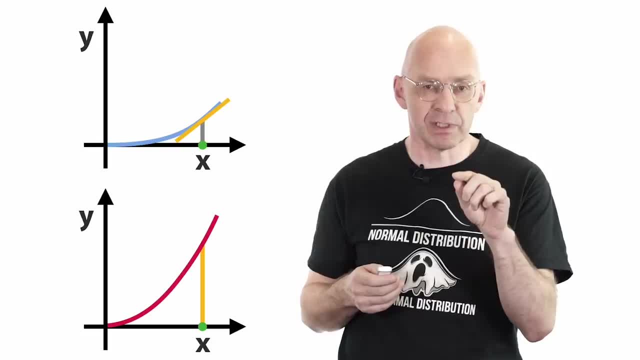 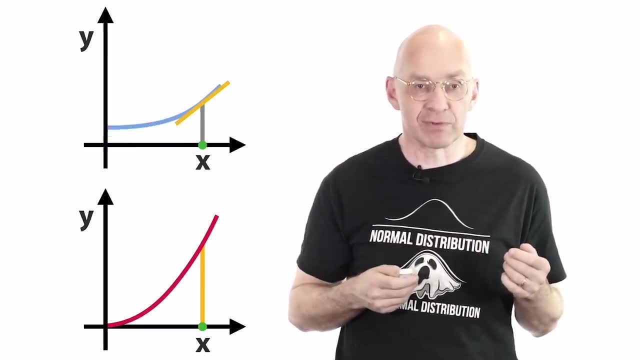 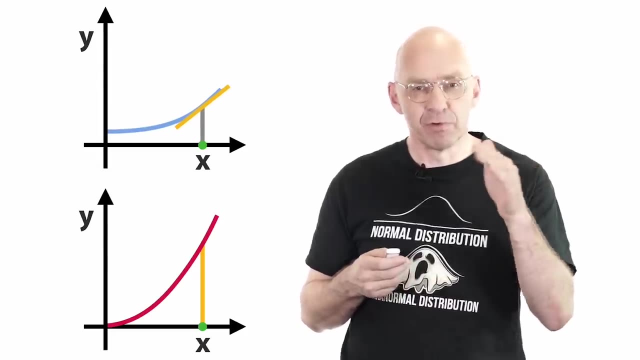 bottom. But if the blue function has this property, then so does every vertical translate of the blue function. Obvious right. All of these guys are antiderivatives of the red function. They all share the same slopes at the same points. Again, the blue function is an antiderivative of the red function, but 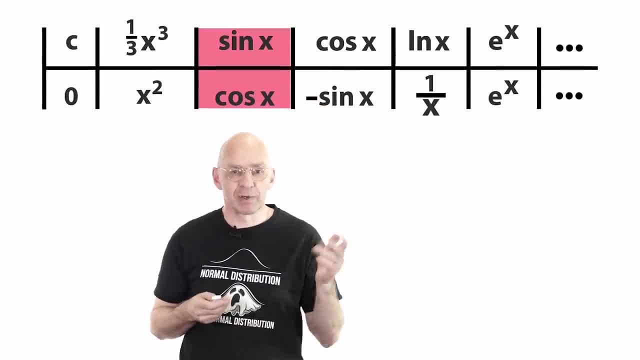 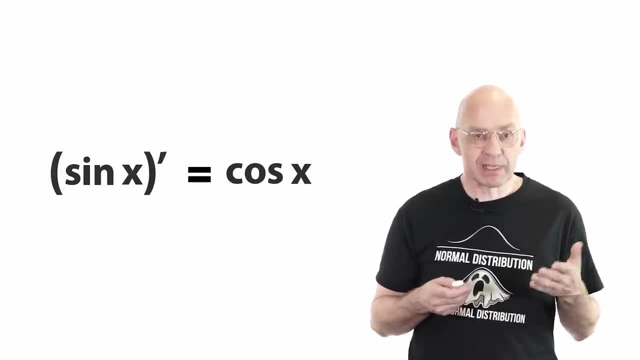 so is every vertical translator. Let's also quickly check the algebra. For example. this entry says that the derivative of sine is cosine, and translating up or down means adding some constant to sine. So can you see that what we see in front of us stays true if you add a constant to sine? Obvious right. 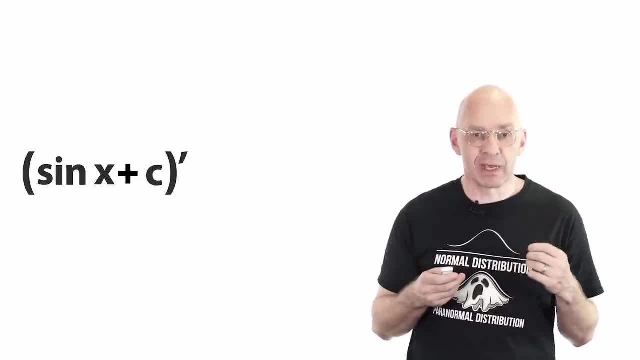 Just unleash the sum rule, which says that the derivative of the sum is the sum of the derivatives. and there we go: Same derivative, Nice. Okay, that was bump number one: The fact that functions have infinitely many antiderivatives and that all these antiderivatives are 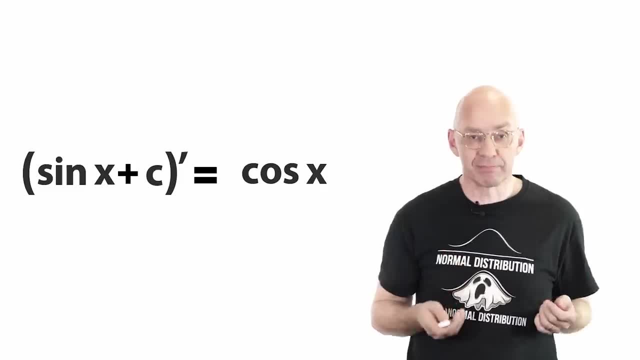 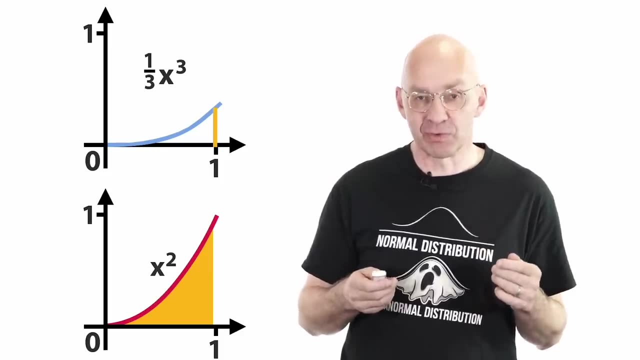 really all the same, up to addition of constants, Just shifting up and down, Not a big deal. What about bump number two? Well, for the antiderivative area calculation up there to work, the top function has to be equal to zero. Add x. 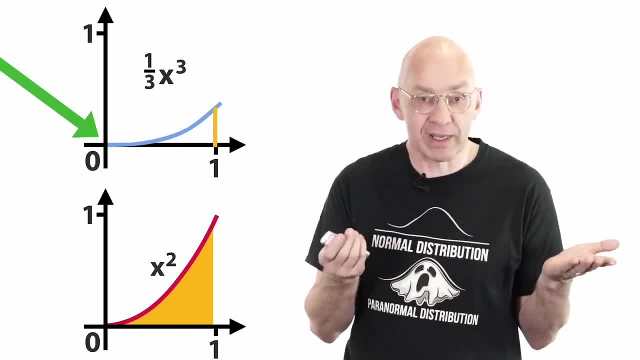 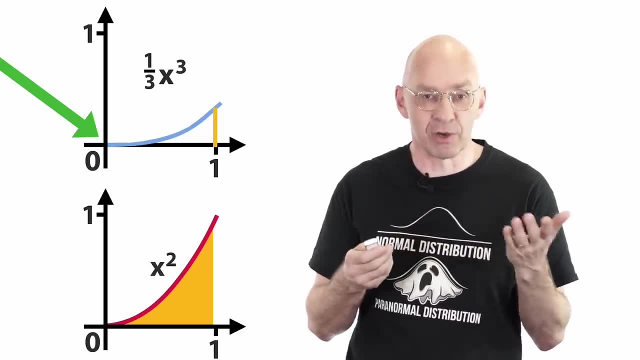 is equal to zero. Right, It's got to be zero there. Why? Well, if we move the right boundary of our area from one to zero, the area shrinks to zero, and so the function on top should be zero at zero. Okay, But now. 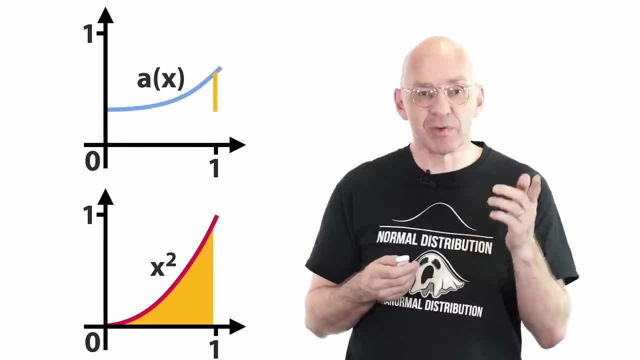 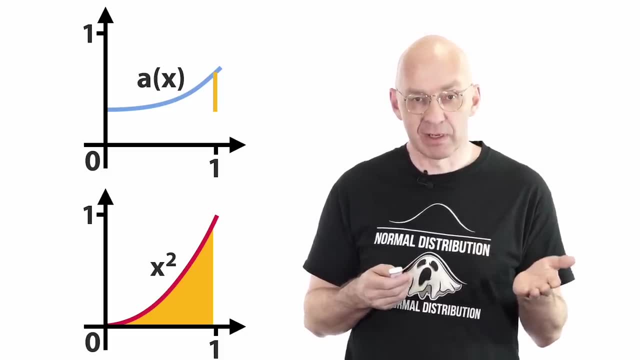 we have these other antiderivatives. How can we use one of these antiderivatives to find the area? Not hard. We know that the area is the length of the yellow segment, but that length is easy to calculate by evaluating our new. 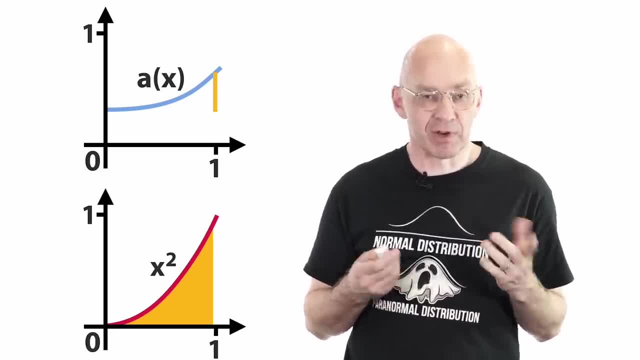 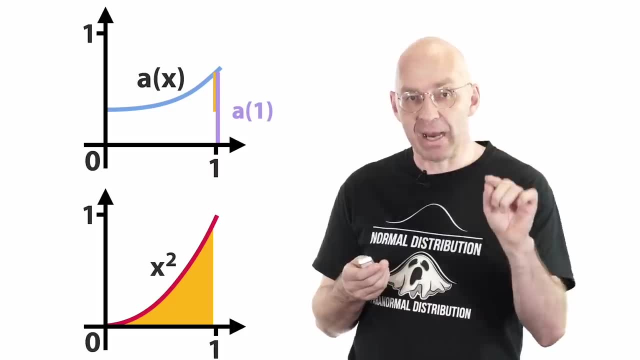 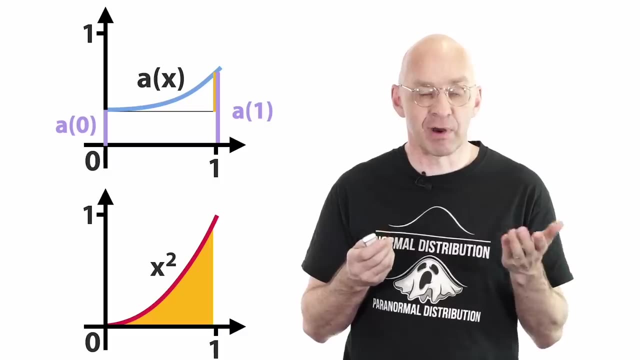 antiderivative at the left and right boundaries of our area. Right, The yellow length is simply our antiderivative evaluated at one minus the antiderivative evaluated at zero. In fact, it's easy to see that this even works if the left boundary is not zero. There, The area between three fourths and one is 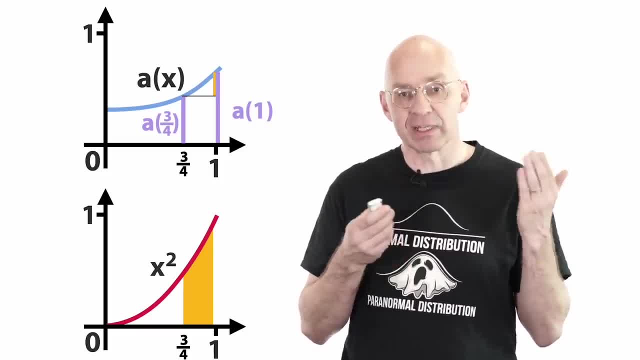 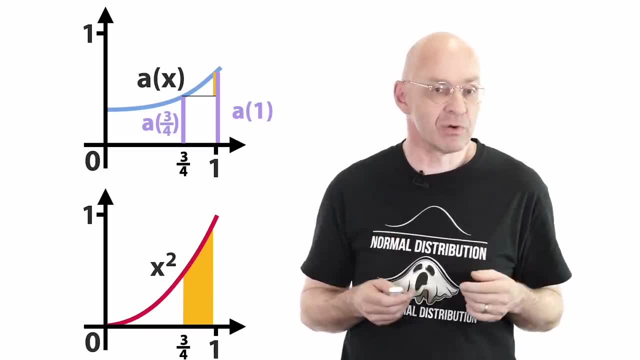 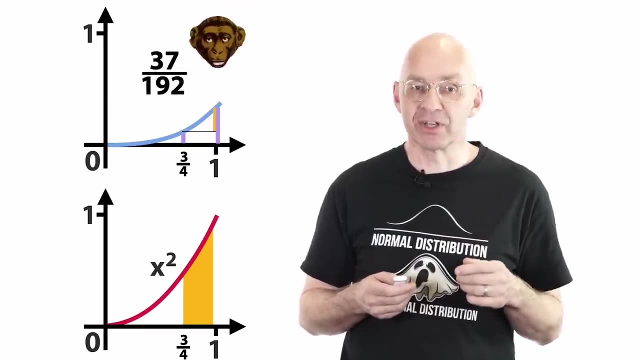 simply the antiderivative evaluated at one minus the antiderivative evaluated at three fourths, And that works for all antiderivatives and so also for the one we started with. And so the area here is this difference, which happens to be 37 over 192.. And if 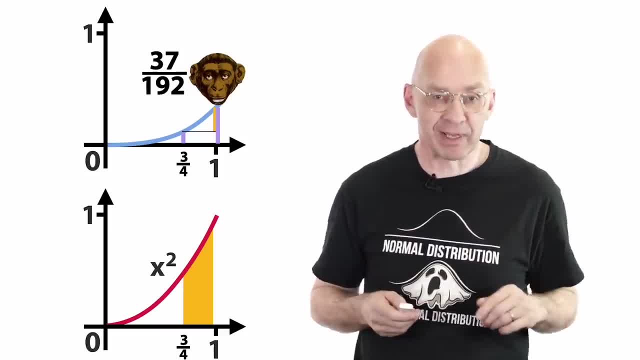 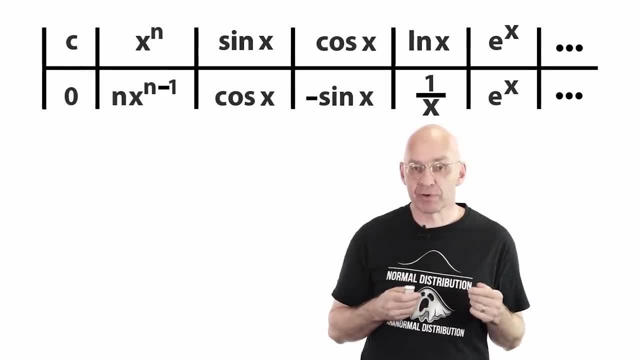 your life depends on figuring out this area. you'll be super happy at this point. Great. Anyway, reading our table from bottom up gives us the antiderivatives of some important functions for free. Now, in theory, we could do much, much more by extending our table into a monster table that features all infinitely many. 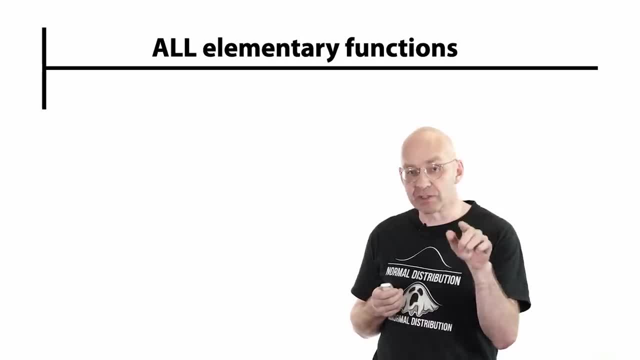 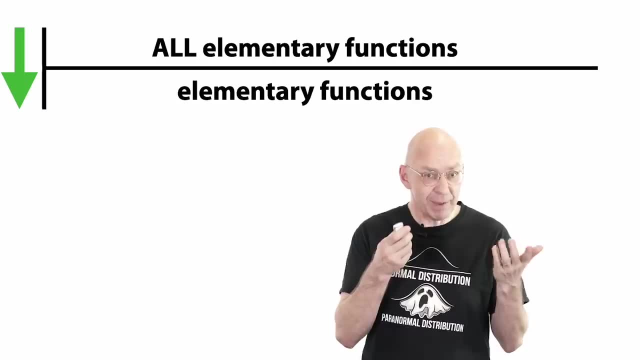 elementary functions at the top, And since all elementary functions have elementary derivatives, the corresponding entries at the bottom would also be elementary functions. And remember, we're talking about infinitely many entries at the top, and so, who knows, maybe we actually also get all elementary functions at the bottom. That 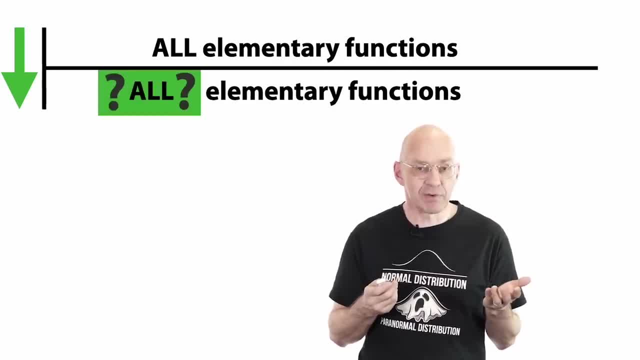 would be great, because if you then challenge me to find the antiderivative of some fiendishly difficult elementary function- f- f for fiendish- then I could look up f at the bottom of my list and find its antiderivative right above Easy right. Well, there are a few tiny problems with. 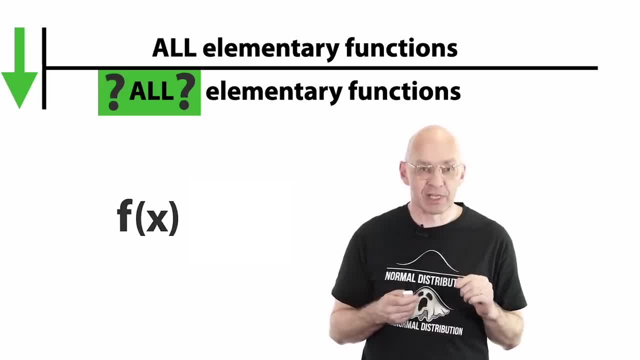 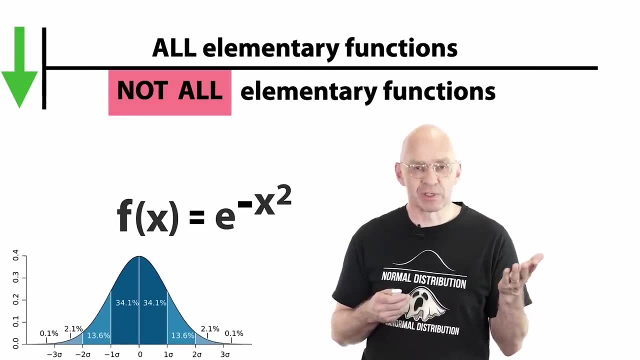 this approach. First, it turns out that there are actually elementary functions that do not show up at the bottom of our list of derivatives, Like this super famous function over there: e to the minus x squared, the function at the heart of the normal distribution, Why not? f is just minus x squared substituted. 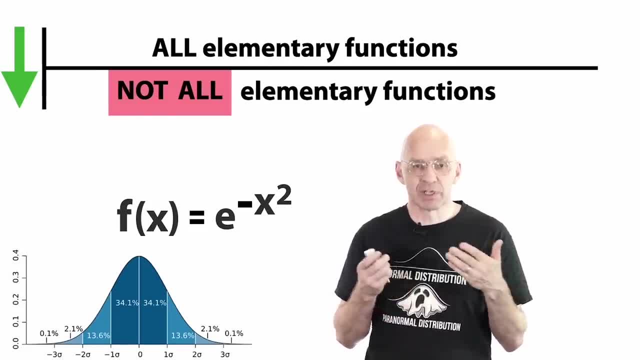 into the exponential function. Basically, one of our atoms substituted into another atom. Simple, No problem differentiating this elementary function using our fifth rule, the so-called chain rule. right A case for our monkey. However, there is no elementary counterpart of the chain rule. 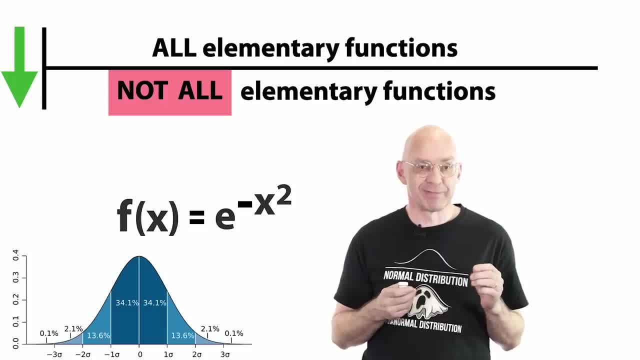 when it comes to finding antiderivatives. Bummer, There are elementary counterparts to the sum and difference rules, but not for the chain rule, the product rule and the quotient rule, And it turns out that the absence of these rules translates into some elementary functions not showing up at the bottom of our list. 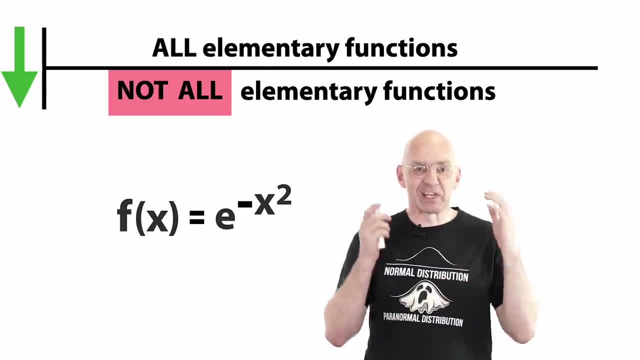 like our fiendish friend. In fact, given a randomly generated elementary function, it's almost certain that it won't appear at the bottom, that it won't have an elementary antiderivative. And there's another problem Because of the absence of these. 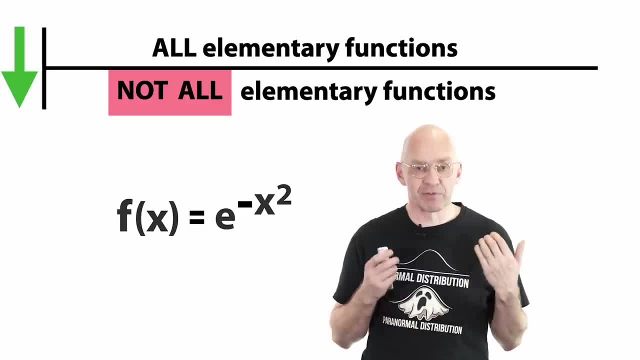 three important rules. it's also not straightforward to determine which elementary functions do have elementary antiderivatives and which don't. For example, to prove that this super famous and super important elementary function over there does not have an elementary antiderivative is crazy hard And even 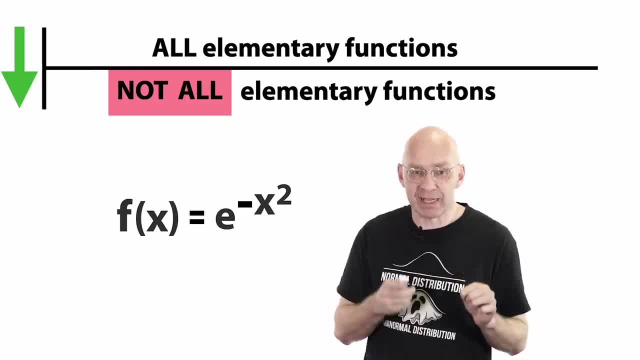 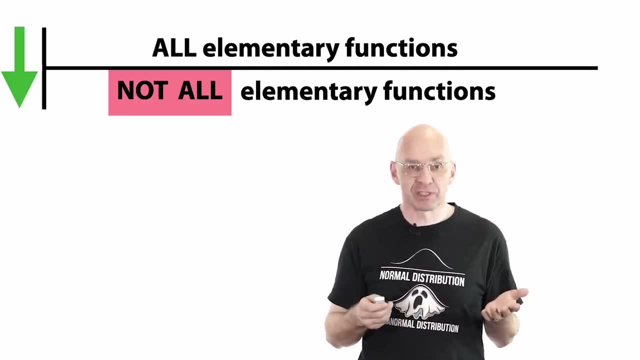 that is not the end of our problems. Even if somebody tells you that a certain elementary function has an elementary antiderivative, it's usually not straightforward to find this antiderivative. In any case, using that table up there in reverse is incredibly useful and powerful in itself. and while those problems we just stumbled across, 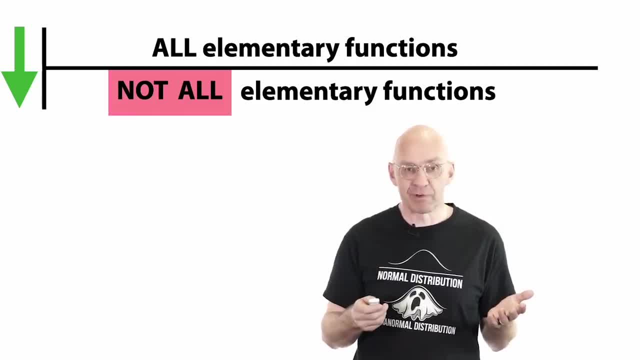 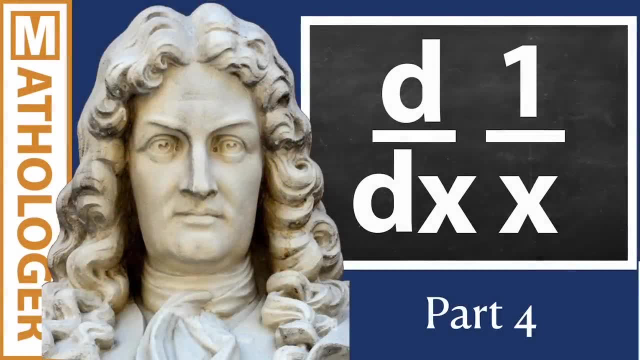 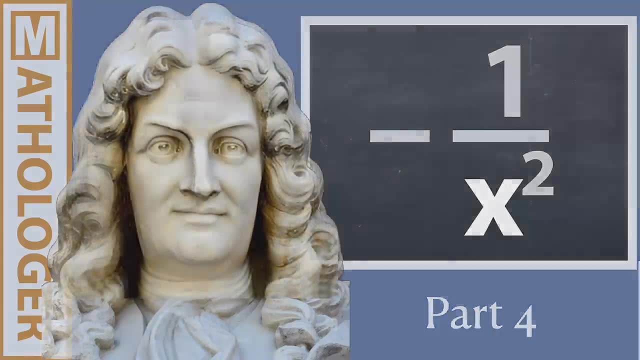 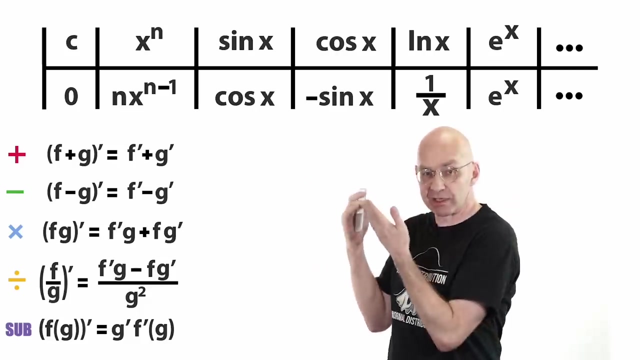 are real problems. there are also lots of tricks to overcome and work around them, But those are topics for another video. All in all, the elementary core of calculus is this list of derivatives up there, plus the rules for finding derivatives over there As a challenge. 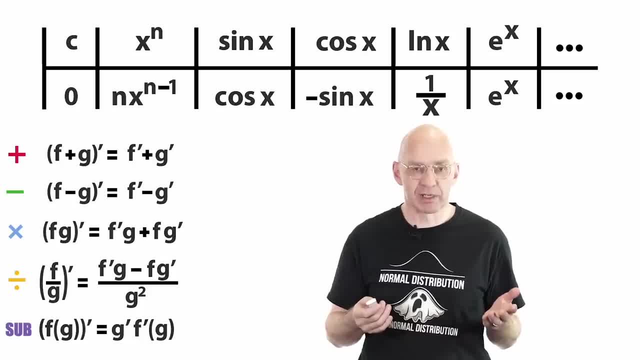 for those of you who know a little bit more, see what adjustments have to be made to what I said so far if we allow taking inverses of functions as a six operations to make new from old functions. Anyway, there is one more aspect to calculus that really makes it unusually user-friendly and that 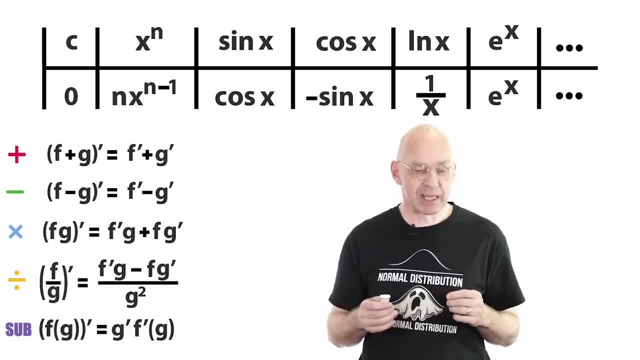 aspect is notation, the nifty way in which we express calculus in symbols. This miracle notation was introduced by Gottfried Wilhelm Leibniz and was further streamlined over the years. This notation allows us to consider the core of calculus as a simple extension of school algebra and, in many ways, the 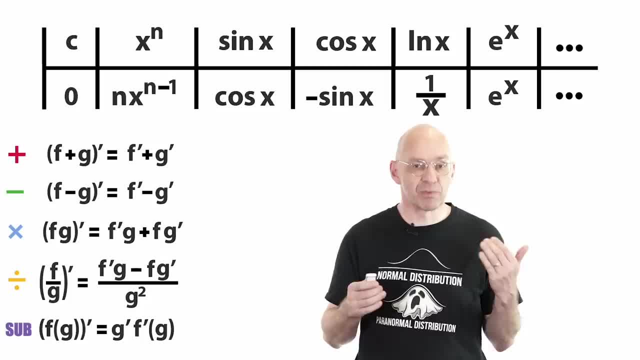 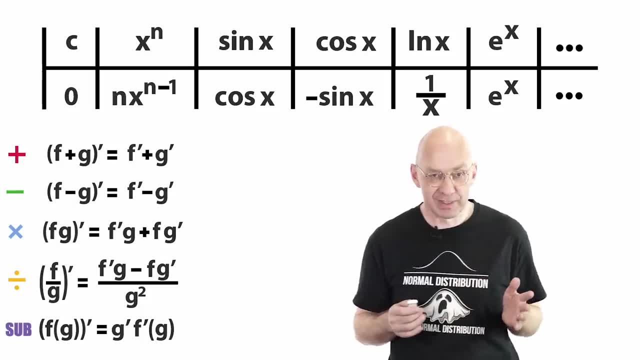 incredible success of that 100 year old calculus book lies in the way it uses Leibniz notation to derive the rules of calculus and to perform calculus. And so, to finish off, let me quickly introduce the most basic elements of Leibniz notation and demonstrate its power by 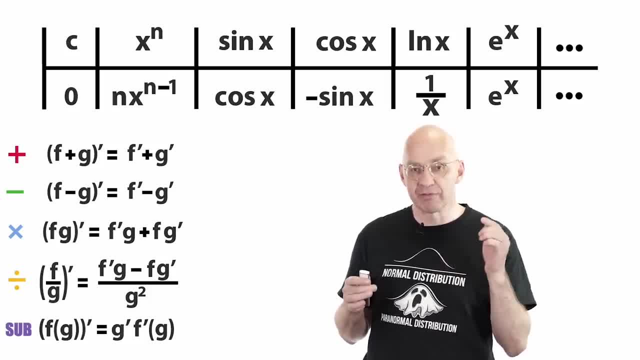 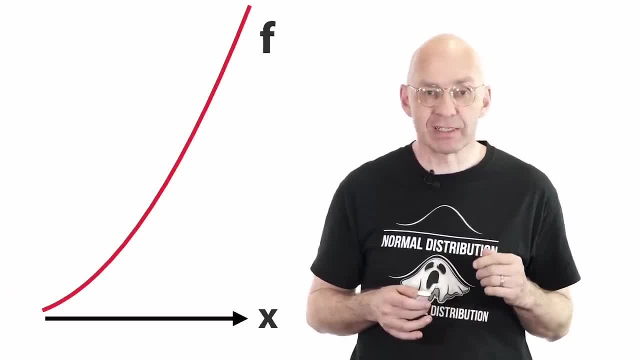 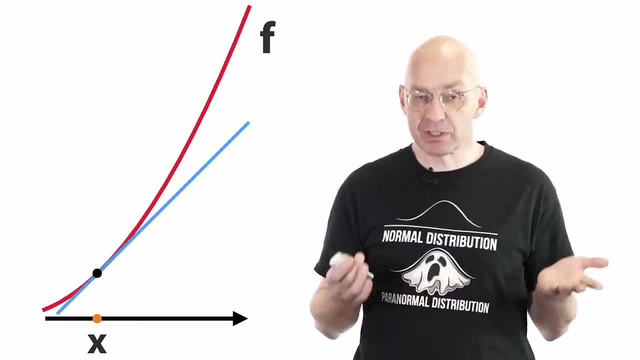 replicating and adding some nice twists to what's done in the book, Derive everything here from scratch in five minutes. Here we go. Calculating the derivative of a function at some point means calculating the slope of this touching line. At first glance it's not clear how we can calculate the slope by 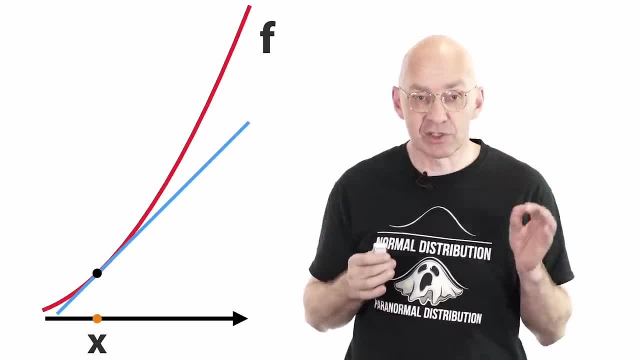 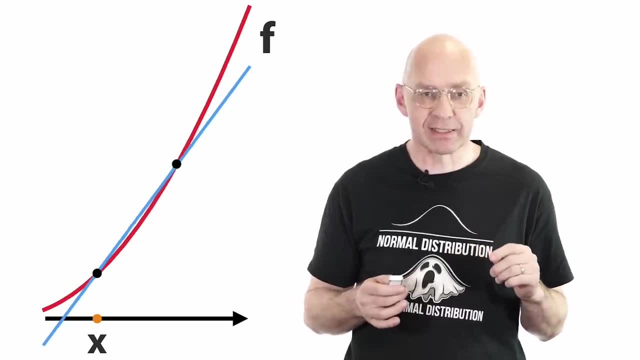 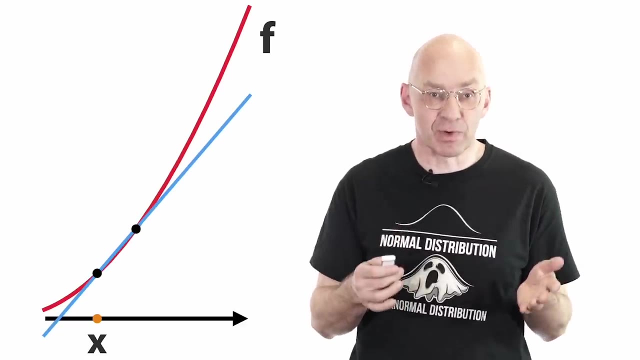 looking at our function. but what's easy to calculate is the slope of a line that cuts the graph in a second point. And now, as you move the second point towards the first one, like this, the slope of the line we're looking at approaches the slope of the touching line better and better. In this way, we sneak up on the 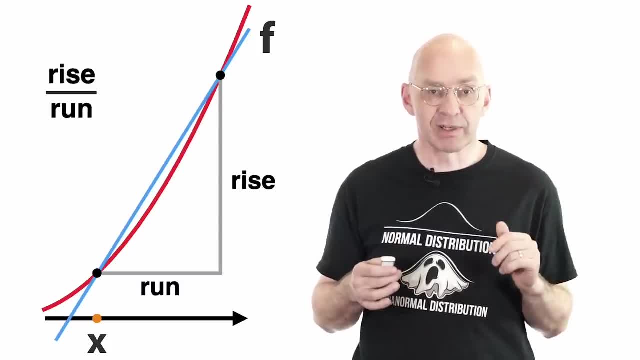 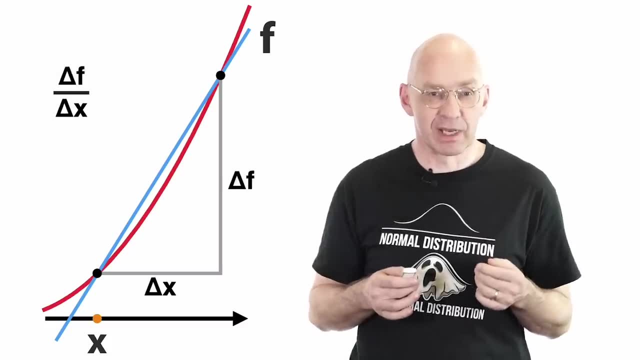 value of the slope that we're really interested in. As usual, we calculate the slope as rise over run. What's the run? Well, some x increment and the rise some f increment. As we push the x increment to 0, the f increment also goes to 0.. 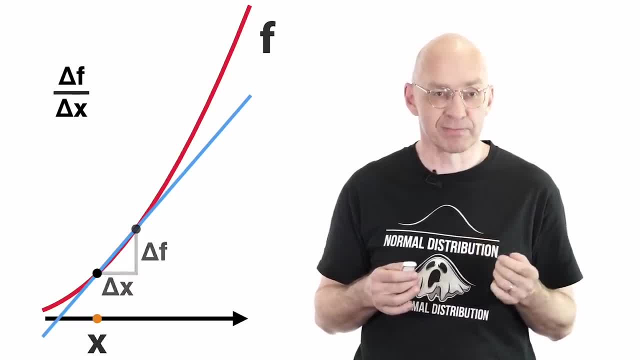 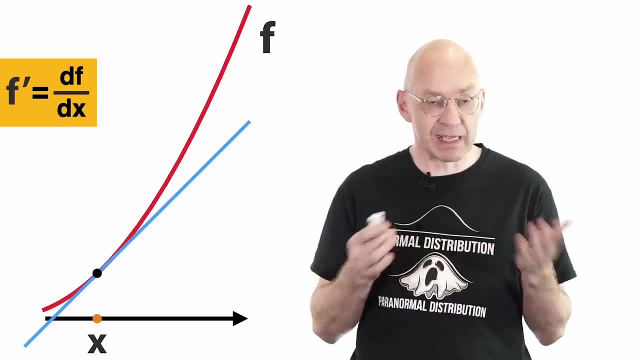 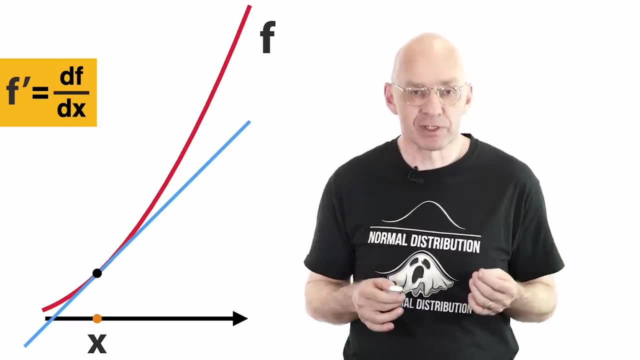 The limiting slope is what we're after, and we write it as df dx. Now, in the first instance, that df dx is just an abbreviation for the limiting process I just described, and by themselves, the df at the top and the dx at the bottom don't appear to have lives of their own. However, the limiting process turns out. 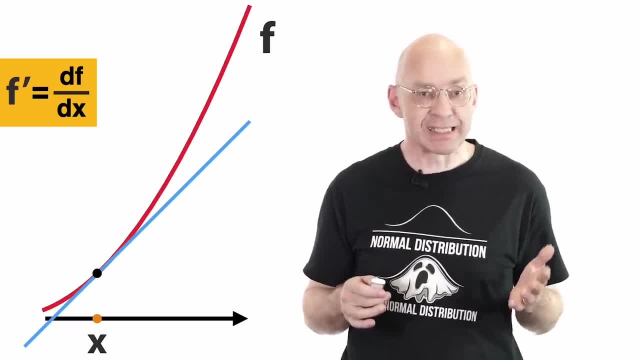 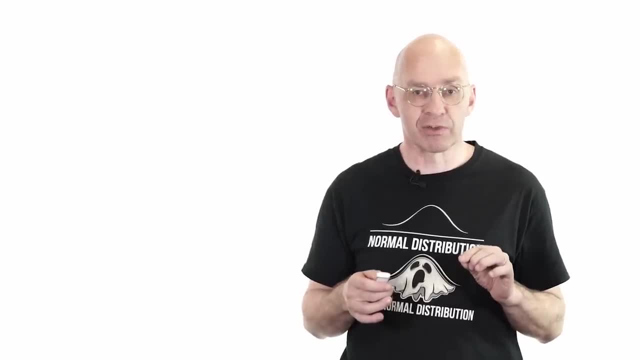 to be such that to some extent we can actually calculate with these d increments very much as with numbers and algebraic variables, And by doing so we can easily get all our derivative rules. It's natural to start with the simple sum rule, but I think it's much more fun. 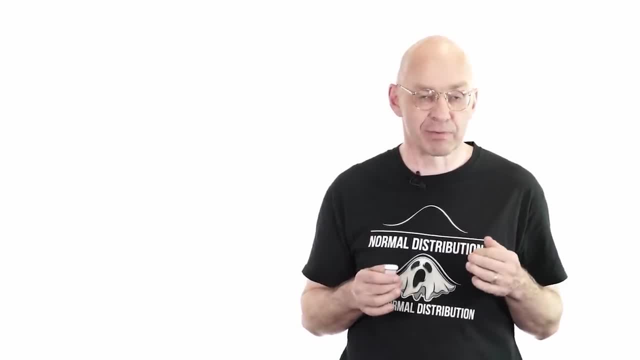 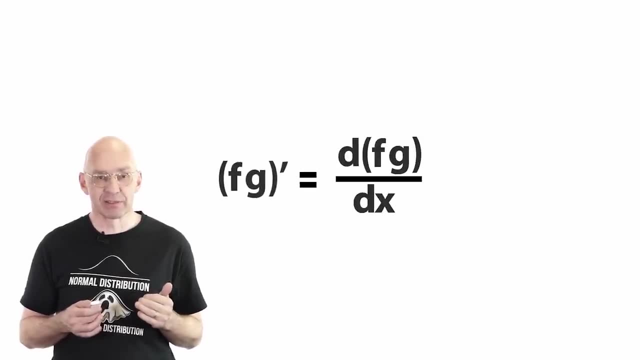 and more impressive, to take care of the more complicated product rule straight away. What's that derivative? Well, in terms of these weird d increments, is this Okay? and what is the increment df times g on top? Well, starting with the product, f times g, as we increment x by dx, f will increment by df and g will. 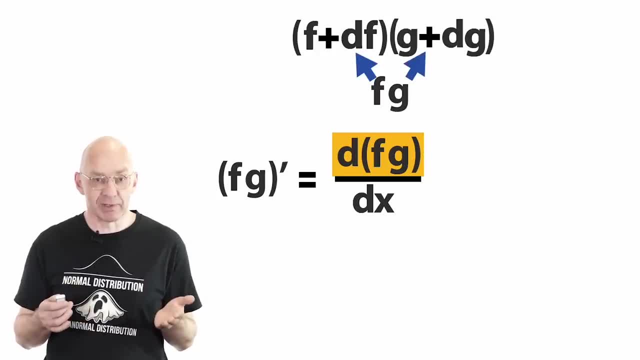 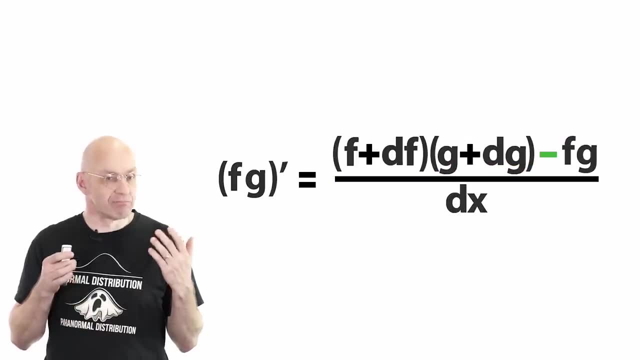 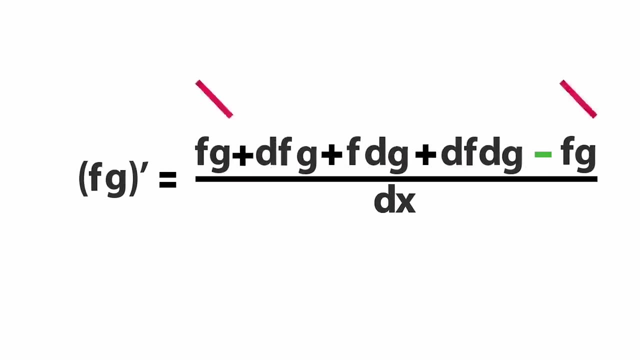 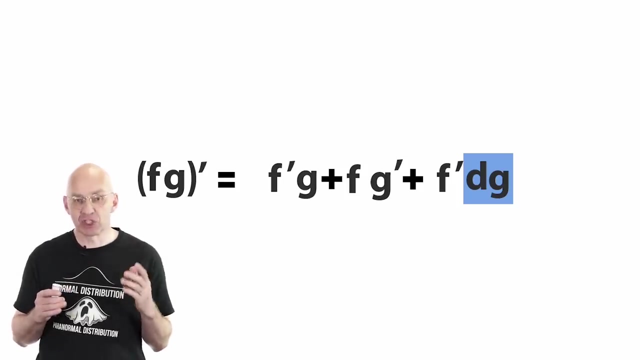 increment by dg. So the orange increment is just the difference between these two products. Okay, but now it's just a matter of algebraic autopilot: Expand the product and so on. Watch and wonder. Now remember, in the limiting process dg actually stands for the G increment. 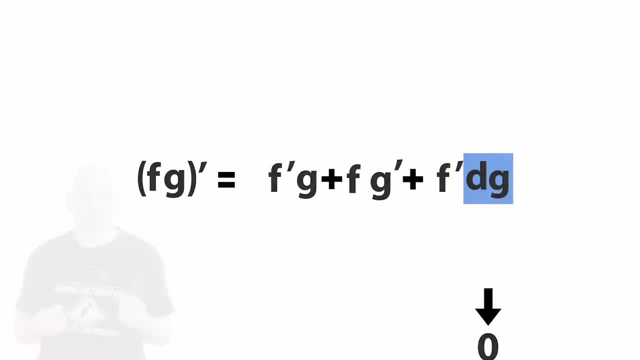 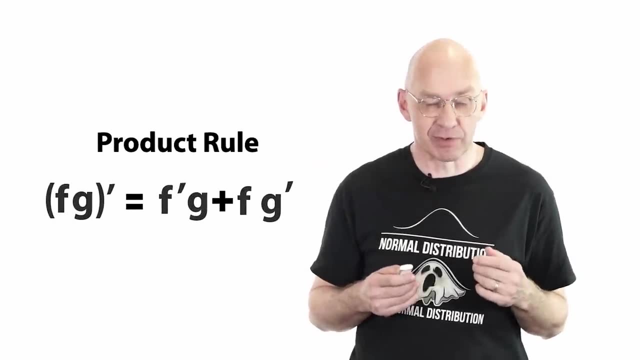 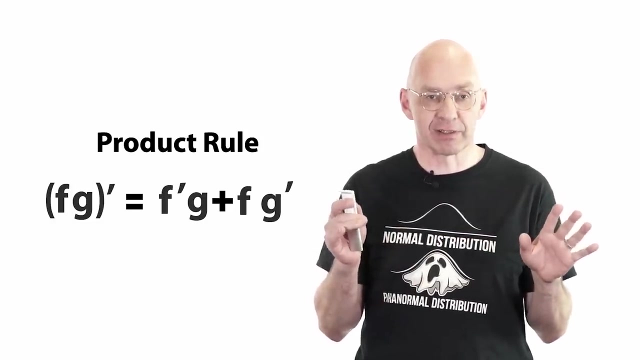 going to 0. And so we can finish our calculation like this. Tadaa, I present to you the product rule. Very nice, isn't it? And now, as promised, I'll animate in derivations of all the other rules of differential calculus and 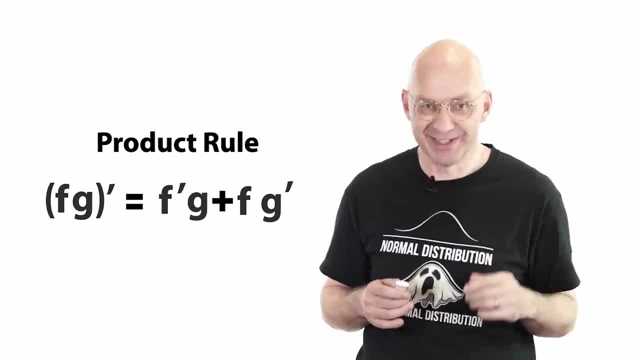 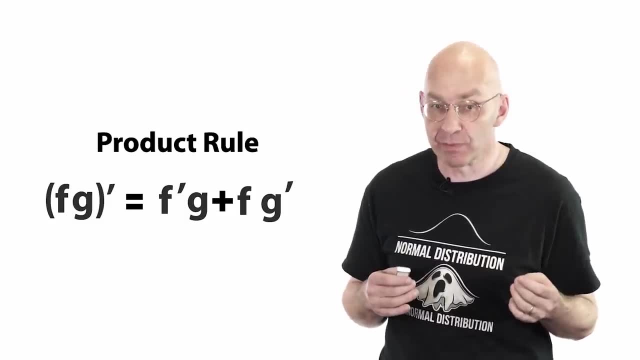 the derivatives of our atom functions, just for you. following this, I'll end with some quick snapshots of a couple of other instances of Leibniz notation working miracles that many of you will be familiar with but that I won't get around to covering today. These snapshots also feature the second main. 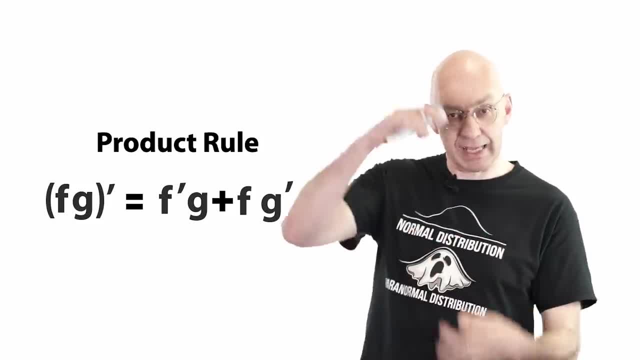 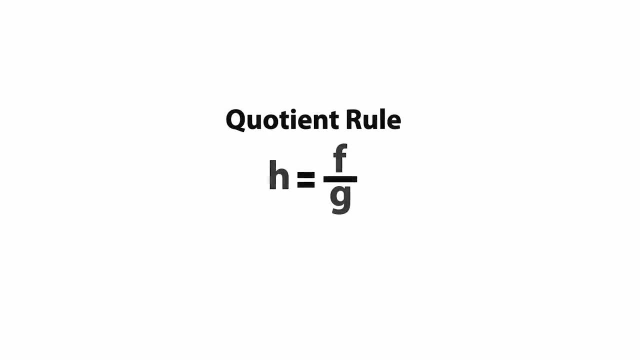 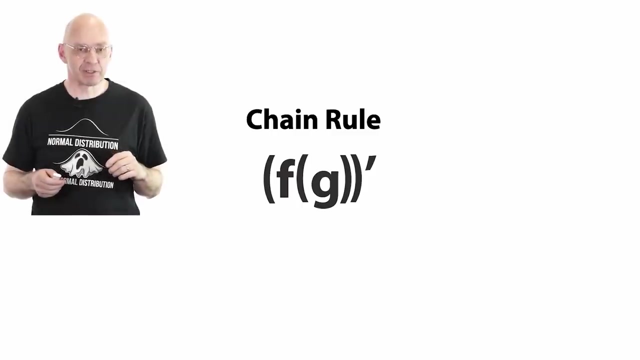 ingredient of Leibniz notation, the integral sign that elongated S Leibniz's way to denote the antiderivative Enjoy, Thank you, Thank you, Thank you. The derivative of one function is subbed into another. What's that? 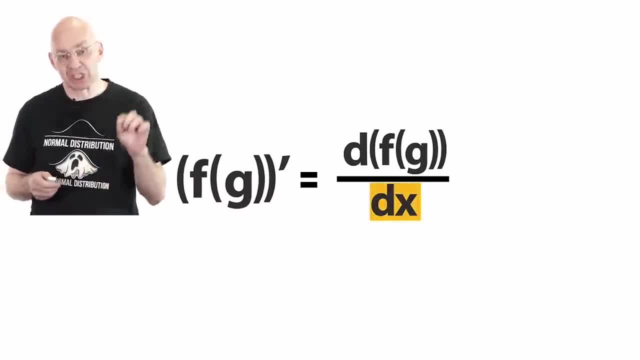 Well, as the variable x changes by dx, the function g changes by dg, And dg is equal to this Right. dx cancels out dg is equal to gg. Now, as g changes by dg, the function f changes by df And df. Well, on the one hand, df, is this Obvious right Again. 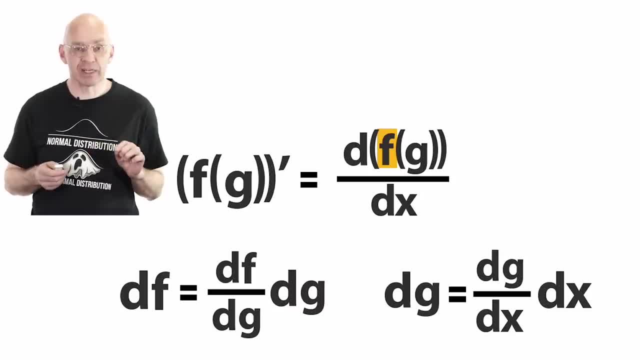 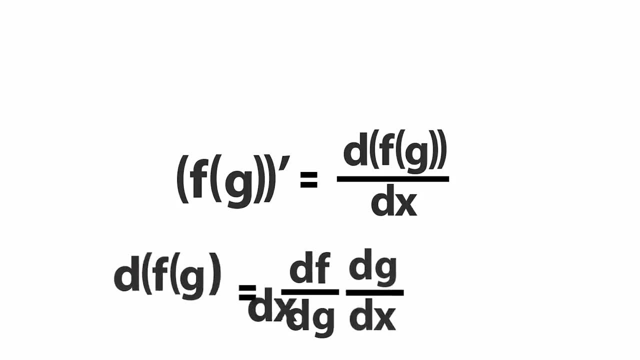 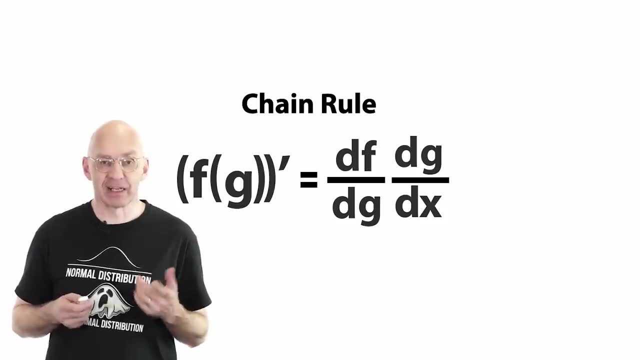 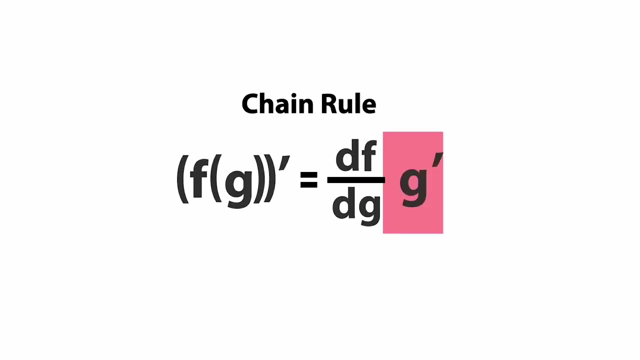 dg cancels. On the other hand, df is really the total change we're after, And now we just go on autopilot. Very pretty, isn't it? Let's chuck the primes in to put this formula in the shape I showed you earlier. 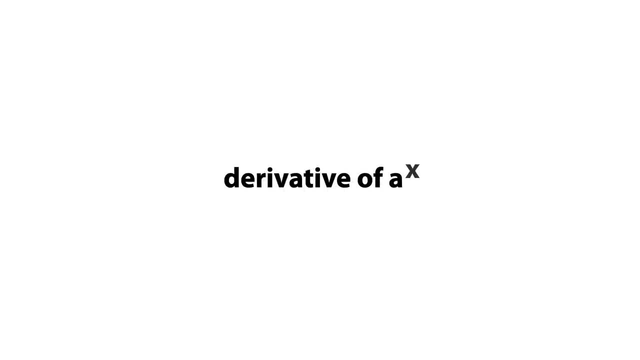 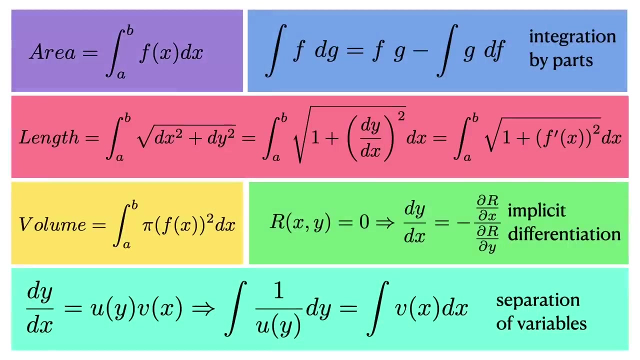 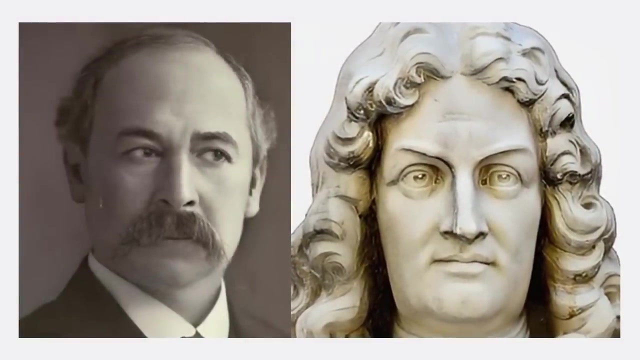 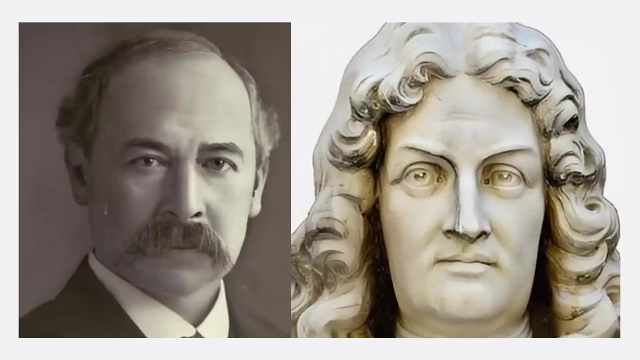 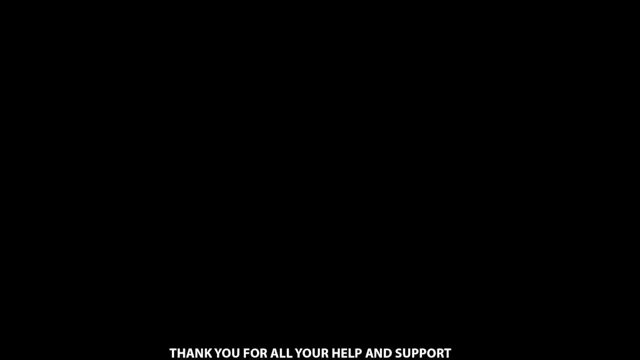 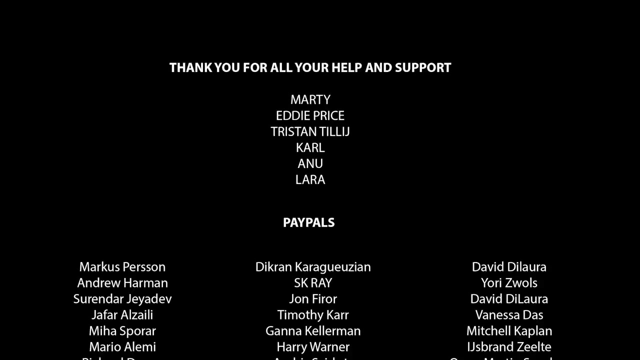 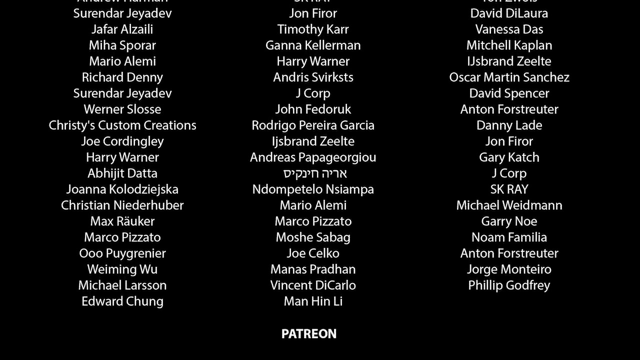 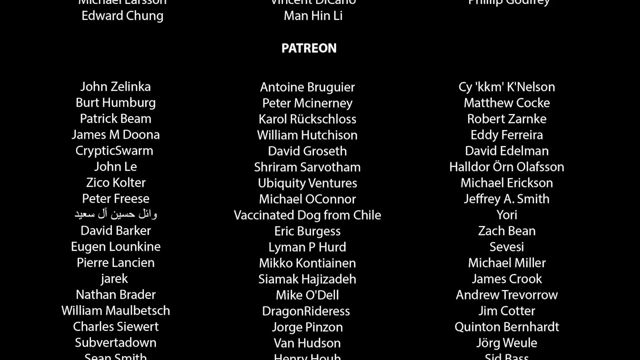 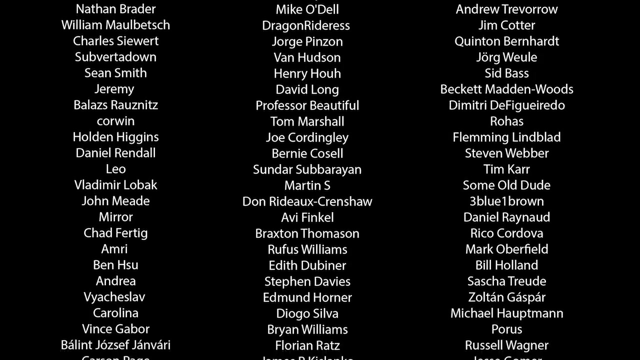 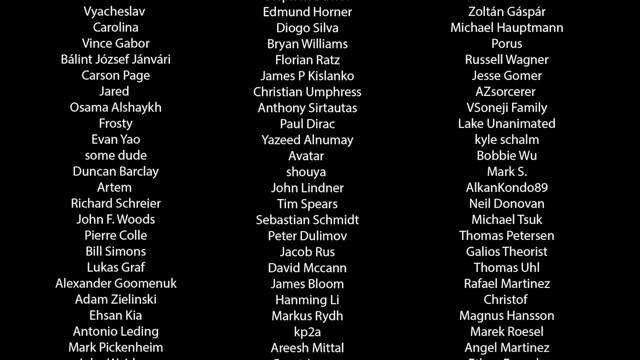